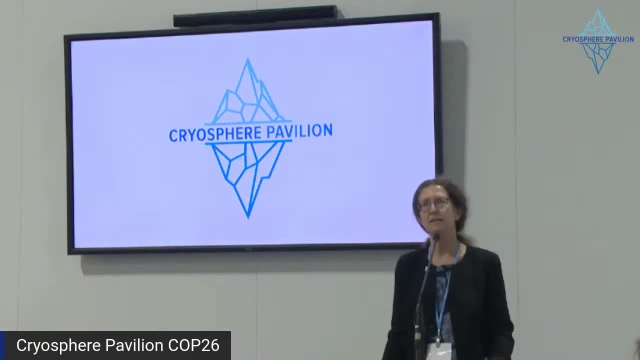 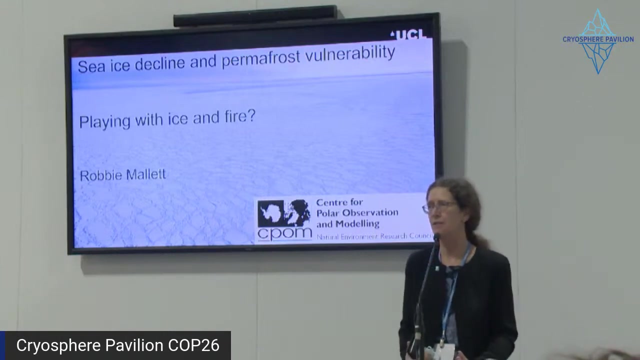 This next event is about one of the complicated issues around cryosphere, because these different elements in snow and ice systems on the planet have a lot of interaction with each other, and that's not always clear. It's something that is an area of active research, but it's one of the reasons why these cryosphere dynamics are so very important as we're aiming for greater ambition. 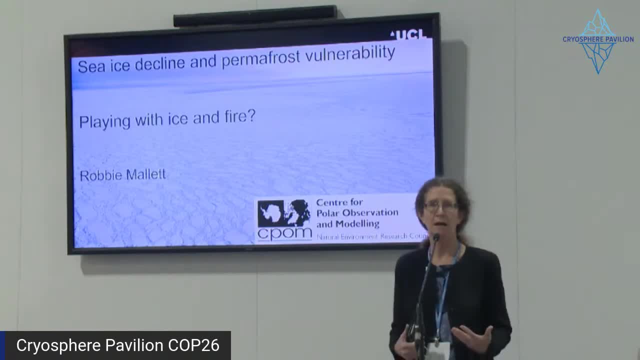 One of the reasons that the 1.5 degrees Paris goal is so very important. So this side event is going to explore the connection between Arctic sea ice loss, which has been ongoing for many decades now, and its impacts on permafrost and sort of the biomes, both on the surface on land and under the water. 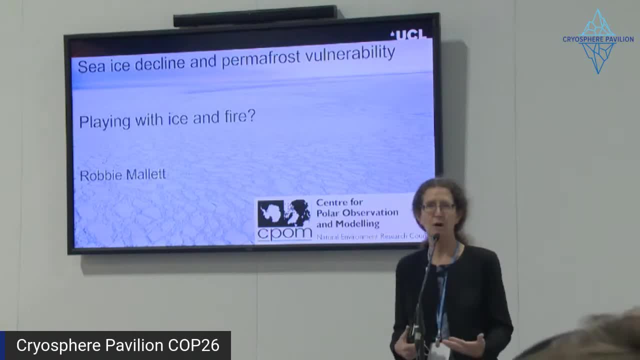 The impacts it will have on subsea permafrost as well as land Permafrost and all of the systems around those. So, again, these are complicated interactions, but there's something that the negotiations do need to take into account as we move forward at the end of this week and especially next. 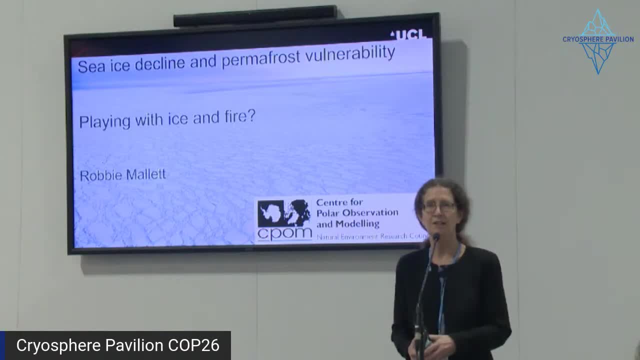 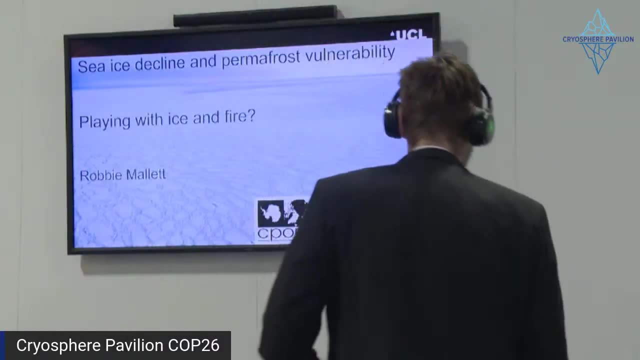 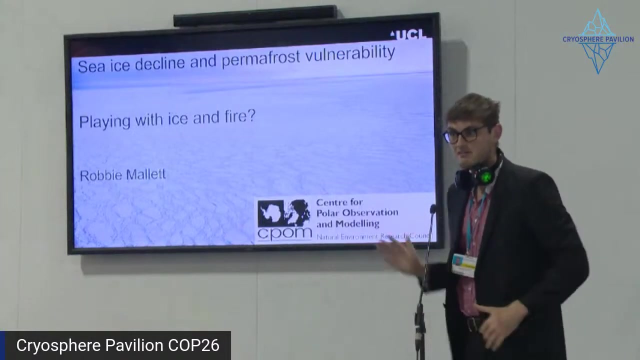 So our first speaker is an Arctic sea ice expert with University College London, Robbie Mallet. Welcome, and we look forward to hearing your presentation, Thank you, Thank you, Thanks, Hi everyone. As Pam said, I work at the Center for Polar Observation and Modeling and I mostly look at sea ice decline, so I'm going to tee it up for Gustav in a minute to talk about the links with permafrost. but one of the real emerging trends that we see, certainly in the last few decades, is sea ice decline in the marginal seas of the Arctic Ocean, and that's really relevant to permafrost because that's where the subsea permafrost lives and also a lot of terrestrial permafrost is being eroded from the coast. 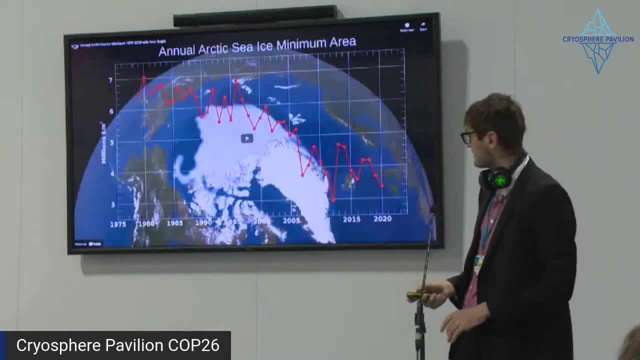 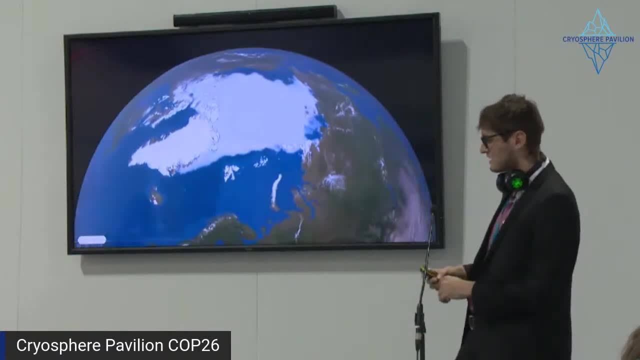 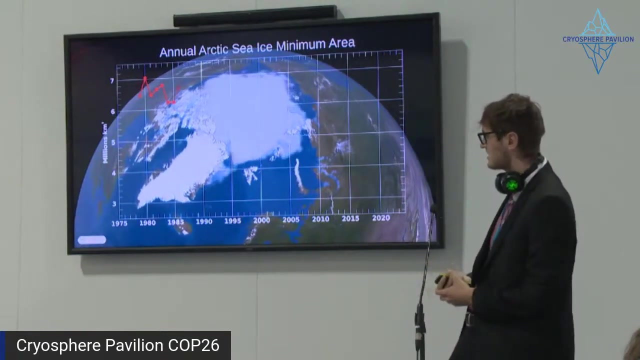 So I'm just going to show a quick animation showing how the sea ice distribution has changed over the last few decades and, as well as looking at the line graph that's going to appear showing the downward trend in the total extent, the total area coverage of the sea ice, it's also really important to pay attention to where we're losing that sea ice. 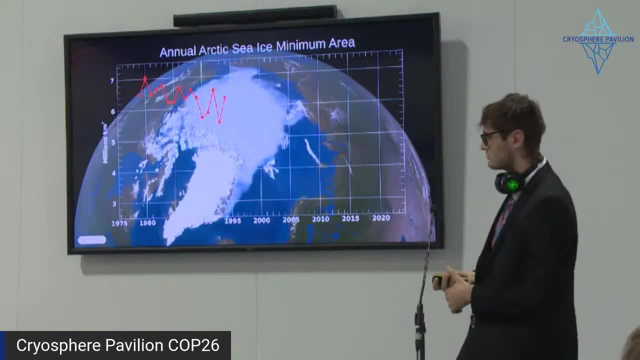 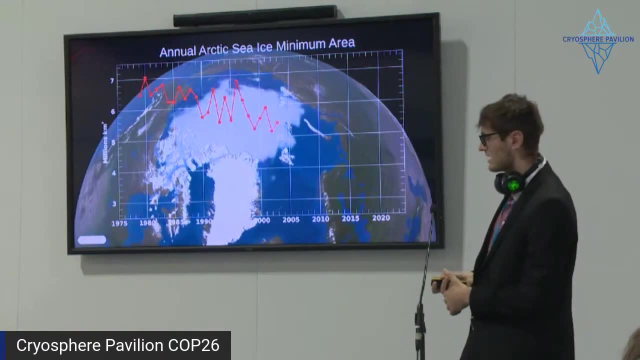 So we're losing it from the northern coast of Siberia, the northern coast of Russia, very, very acutely, And that's exposing the coastline to wind erosion, to Yeah Yeah. It's also exposing the coastline to waves, increased storminess and warming water. 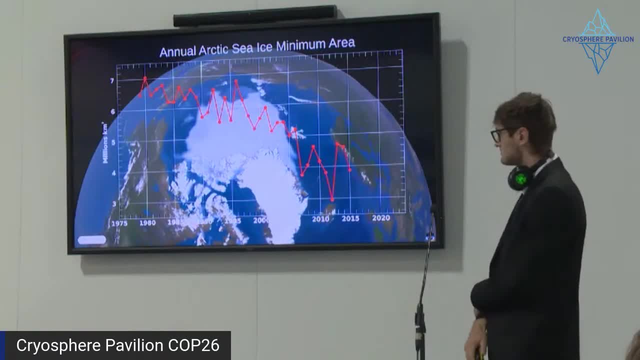 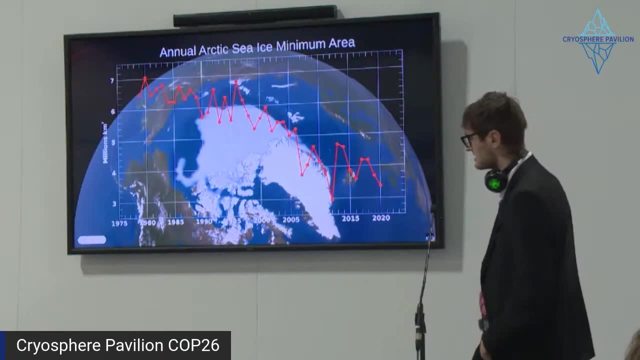 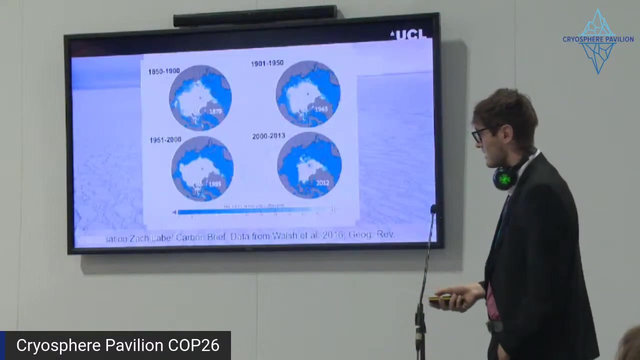 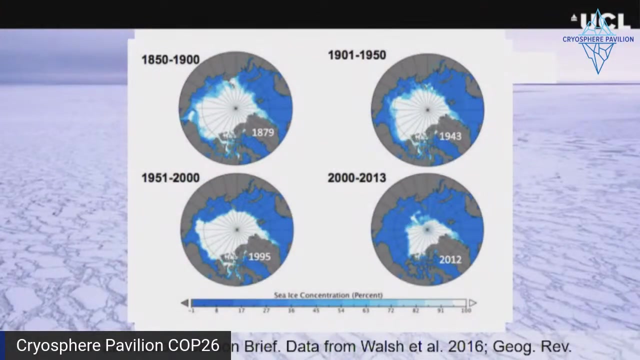 So you can see that the north coast of Siberia there is basically ice-free in summer now and that's causing rapid change in the shelf seas that we see there. Yeah, So that's a similar figure based on some longer timescale reconstructions of the sea ice distribution. that shows a similar trend. 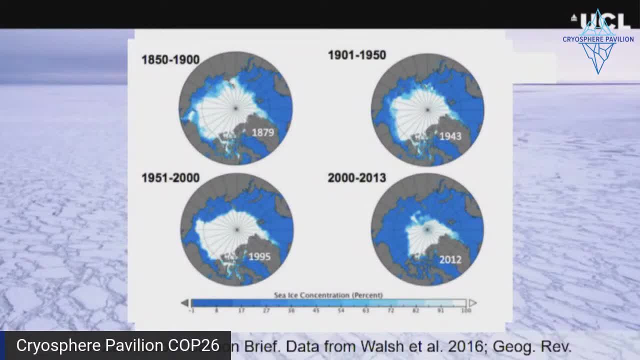 Much more water is being exposed in summer- I should say this is the October sea ice extent- Much more open water, which increases the fetch, That's the distance that the wind can flow over the surface of the ocean and generate waves, And it also increases the surface through which heat and moisture and momentum is exchanged between the ocean and the atmosphere. 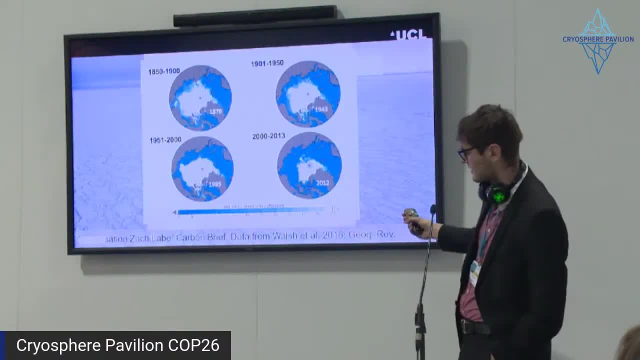 So our most recent period that's included in this reconstruction- we see a really very, very small area of summer sea ice, mostly located north of Greenland and the Canadian archipelago. That's just not protecting the north coast of Alaska and the north coast of Siberia. 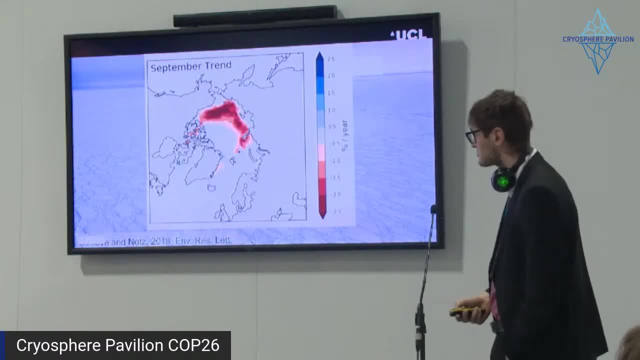 And here's a more rigorous demonstration of those trends. So the trend in September: sea ice from Struve and Notts 2018.. You can see that the trends that we see in the distribution of sea ice in red, that's minus two and a half percent concentration. 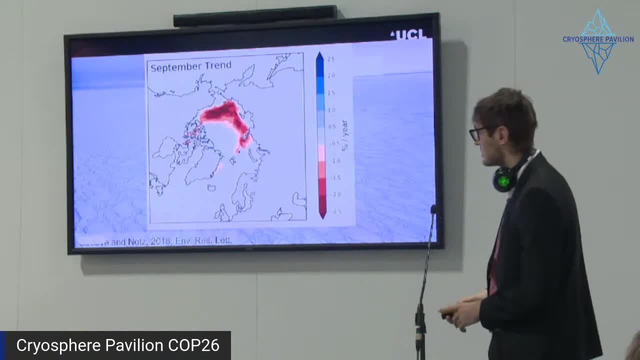 that's the ice coverage in a grid cell per year- is located in these marginal seas of the Arctic Ocean, where we see the subsea permafrost and where we see the ocean interfacing with terrestrial permafrost, And there's a striking similarity. 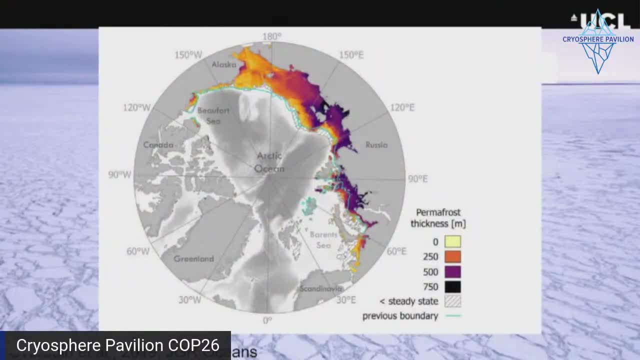 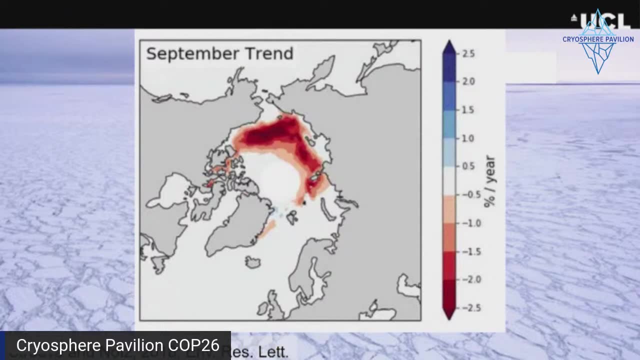 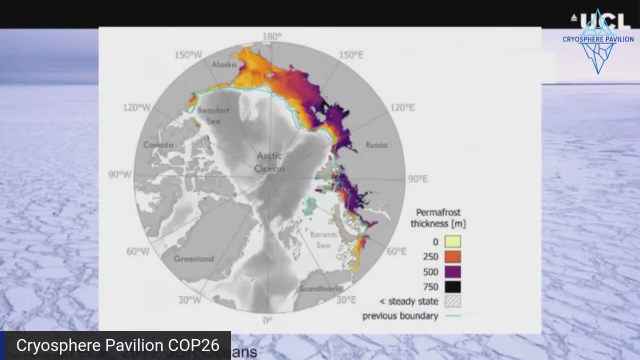 I'm just going to flick back and forward between recent work which shows the distribution of subsea permafrost and where we see the sea ice retreat. So these are completely different, Coincident and related environmental phenomena And we need to pay attention to the linkages between the two. 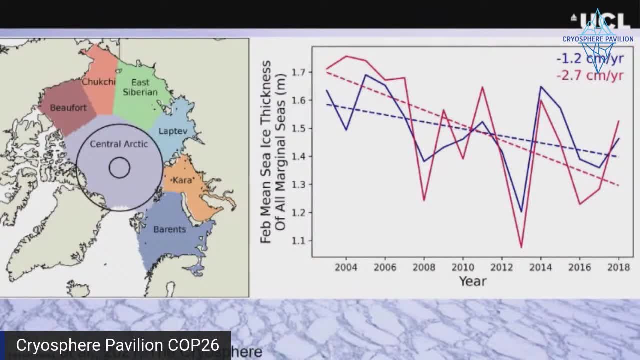 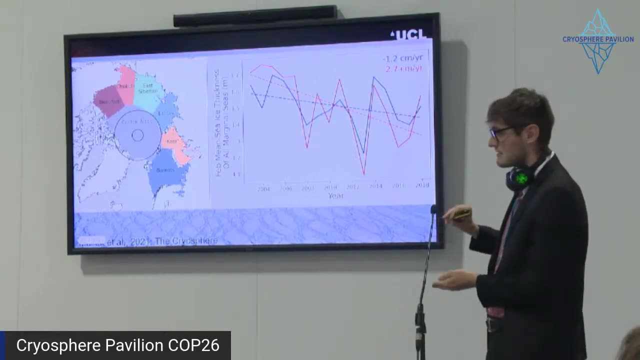 As well as physically retreating the area coverage from the edges of the coast, we also see a thinning of the sea ice. that's really important because even when the sea ice is covering the water, we see exchanges of heat and even wave action. 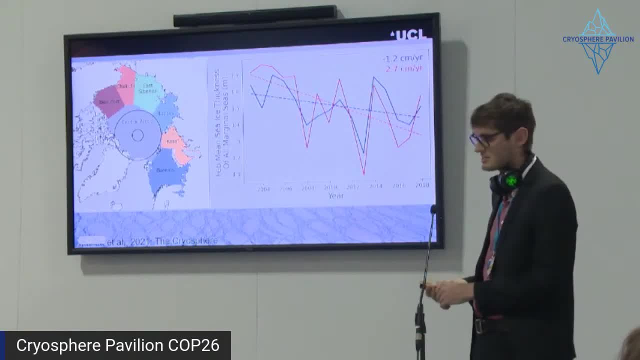 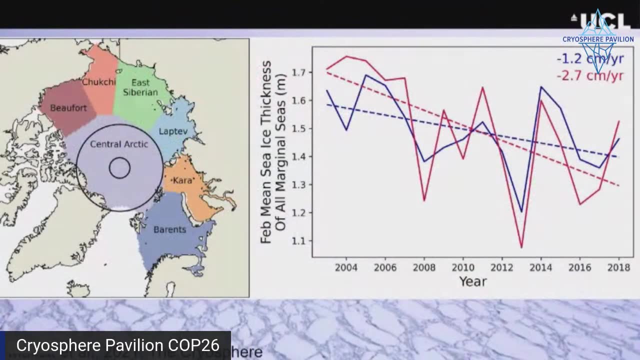 And underneath the sea ice. the waves from the ocean can penetrate the sea ice and be whipped up between the flows, And recent work that we've done at the Center for Polar Observation and Modeling indicates that sea ice in these marginal seas and the marginal seas we characterize as the ones outside the Central Arctic, outside the outermost black circle- 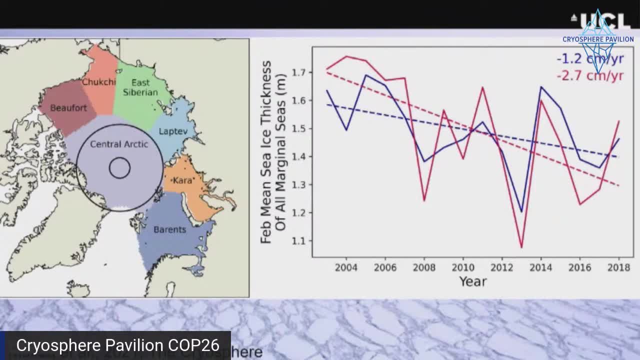 is thinning actually twice as quickly as we previously calculated using satellite data. So there's still a lot of uncertainty. As you can probably see from this plot, there's a lot of inter-annual variability in the sea ice thickness of these marginal seas. 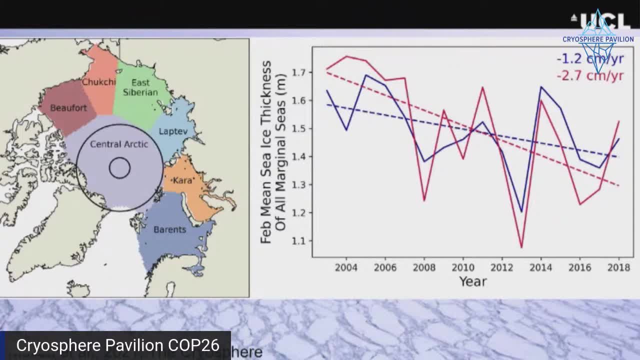 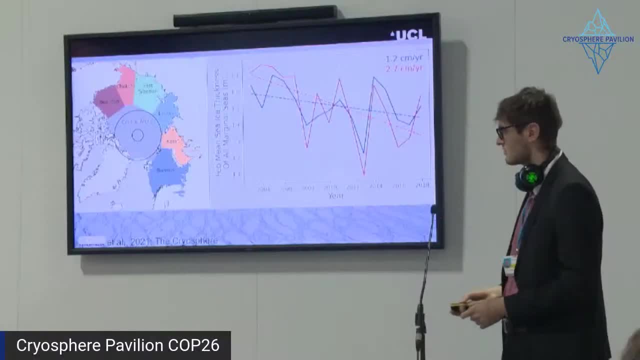 The red line and the red trend is our revised estimate, which is certainly a lot steeper in decline than the blue line and the blue trend, which is the conventionally derived information. And once again, you can see that these marginal seas for which we calculate this graph, 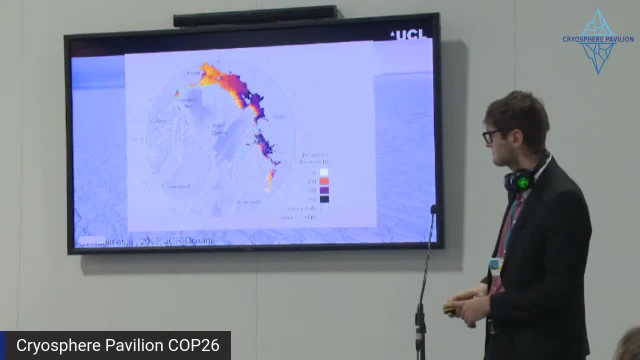 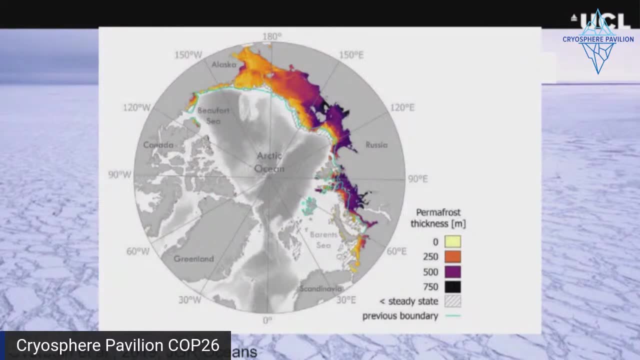 are basically coincident with the distribution of subsea permafrost. I should say also, when the sea ice thins, even though it's providing a physical cover, that heat that's still exchanged between the atmosphere and the ocean in summer has profound effects on the mixed layer, the surface layer of the ocean. 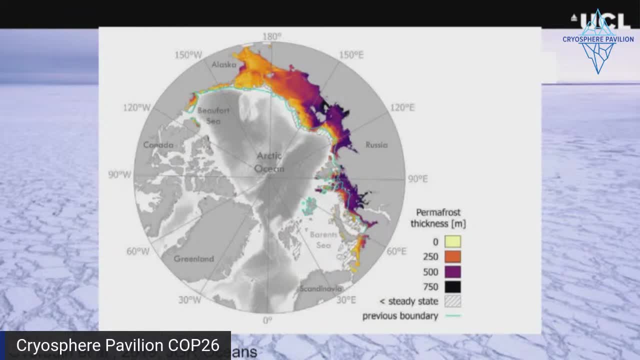 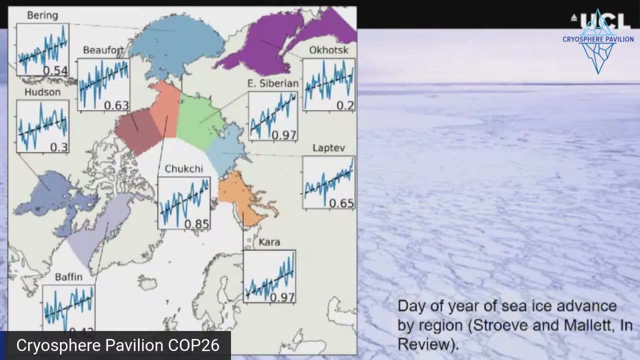 And that is changing the oceanography of these very shallow shelf seas, certainly north of Siberia, And finally compounding the aerial reductions in the sea ice cover and the thinning of the sea ice cover. we also see much longer open water periods. 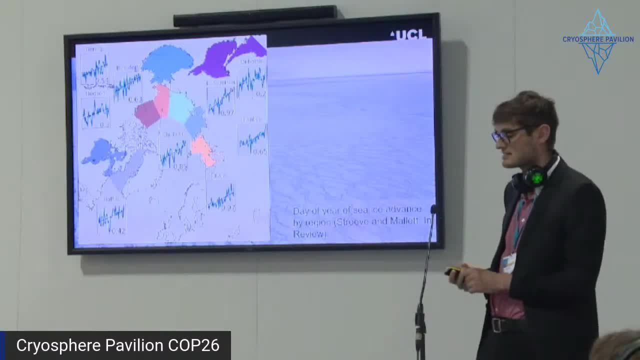 In these regions. So here we're showing the day that the sea ice begins to advance, or actually the day that sea ice advances in full swing in each of these marginal seas And there's a very obvious linear trend in a lot of these seas. 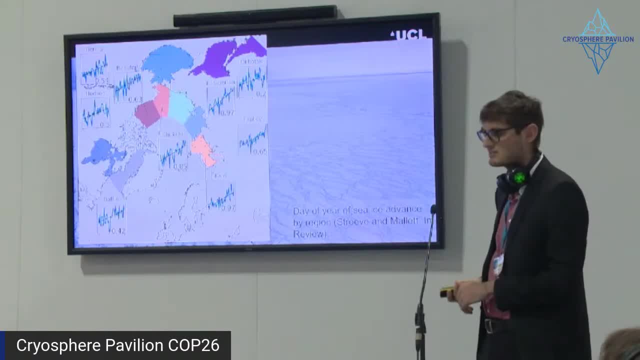 And they show later and later in the year they get the protection of the sea ice from the wind and the waves. So there's a lot happening And you can see this. even though there's variability, that linear trend is very robust And looking at places like the Kara Sea, 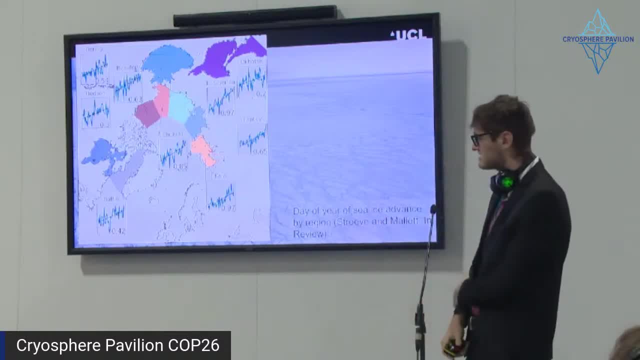 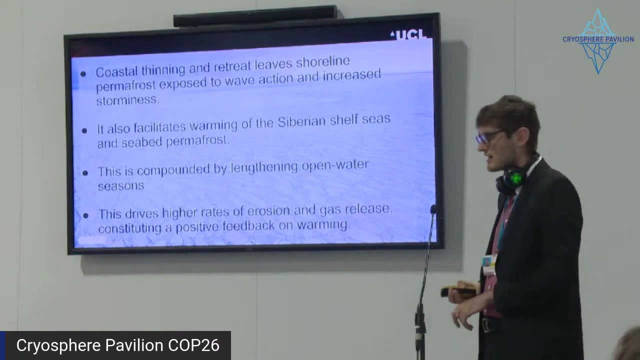 this orange region, we're seeing, almost a day per year later, sea ice advance. So it's radical change in these permafrost filled regions. So just to summarise, we have thinning but also retreat of the sea ice where it exists already. 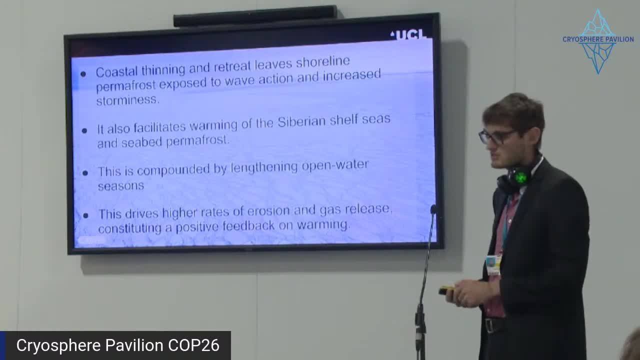 And that's facilitating both oceanographic changes but also changes to the erosion of the land, permafrost, the terrestrial permafrost, which is compounded by longer open water seasons, And I've shown you a graph of the day of sea ice advance. 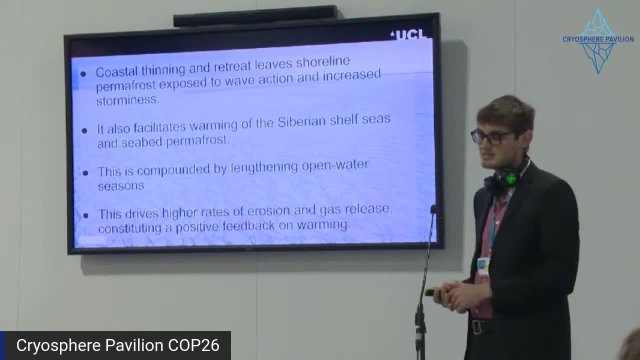 but that's essentially mirrored at the beginning of the season by the sea ice melt onset and the sea ice retreat. So the open water season in these areas is extending both at the end and also at the beginning, And that drives higher rates of erosion and gas release from the permafrost. 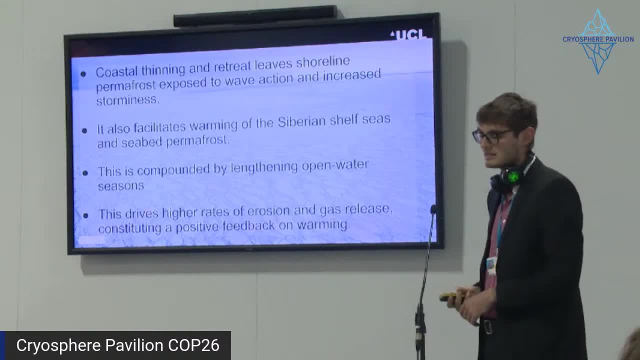 And that's a positive feedback on global warming. So we see sea ice loss driving increased permafrost thaw, which drives further warming, which compounds the sea ice loss. There's been some work looking at what's going to happen in these regions in the future. 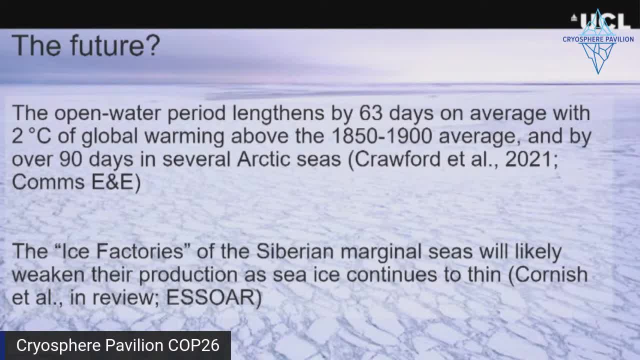 Some recent work using the CMIP6 ensemble showed that the open water period is going to continue to lengthen, which is intuitive but also important to quantify. And even for two degrees of global warming, we're going to see a radical lengthening of the open water period by 63 days and up to 90 days. 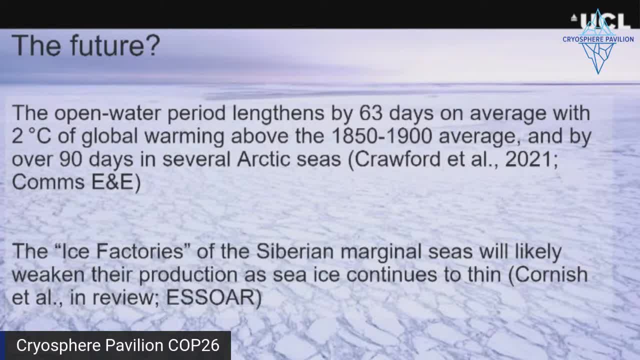 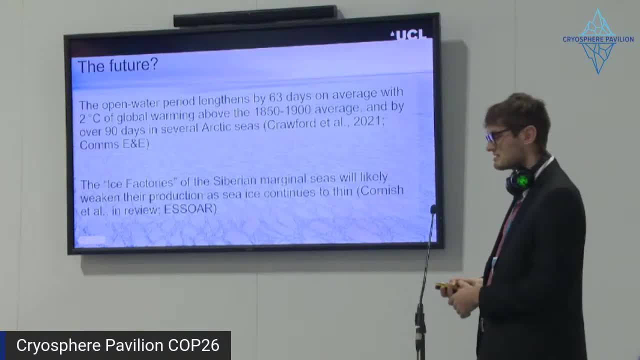 It says, in several Arctic seas, but these are really the marginal seas that interact so strongly with the permafrost. We're also seeing changes in the ice production in these marginal seas. A paper we have in review that I collaborated on recently looked at the Kara and the Laptev seas on the north coast of Siberia. 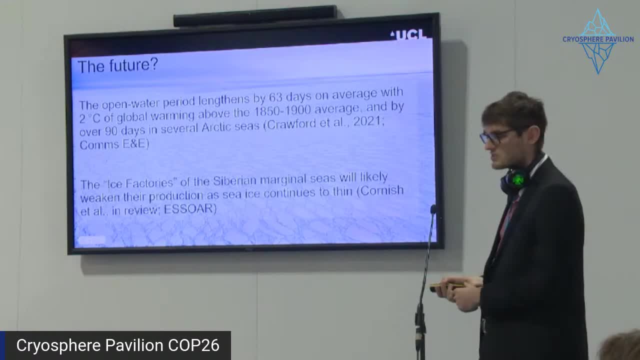 kind of towards the European side And we're seeing ice production is in the future. looking at the CESM large ensemble- So the same model run many times to fully capture the internal variability- We see that the ice production there is going to begin to rapidly decline essentially. 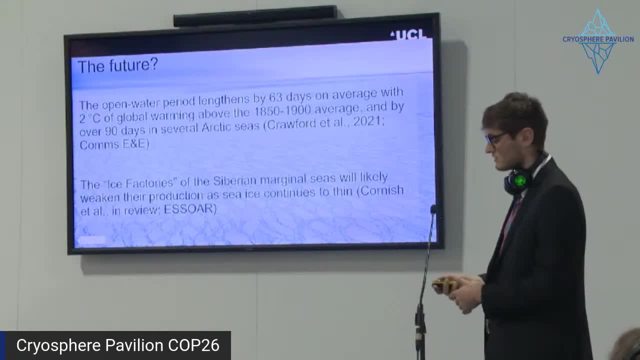 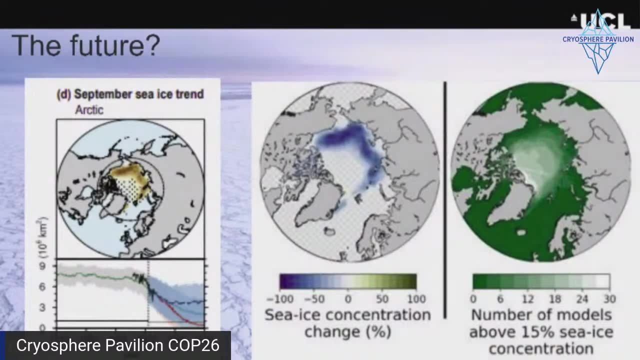 That's going to affect the way that the atmosphere interacts with the permafrost. I've got some low resolution pictures from the not fully released AR6 publication that so many people are talking about this week And they basically show the same story Into the future. on the right you see SSP, the 4.5 radiative forcing. 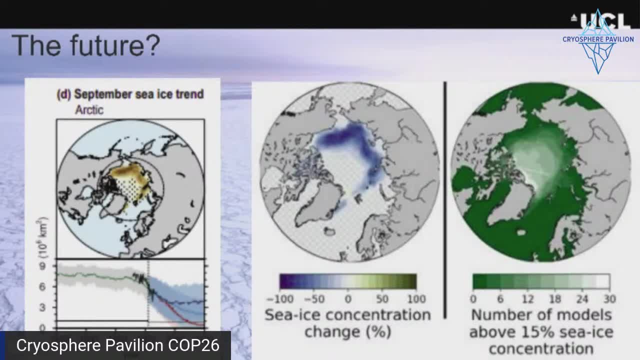 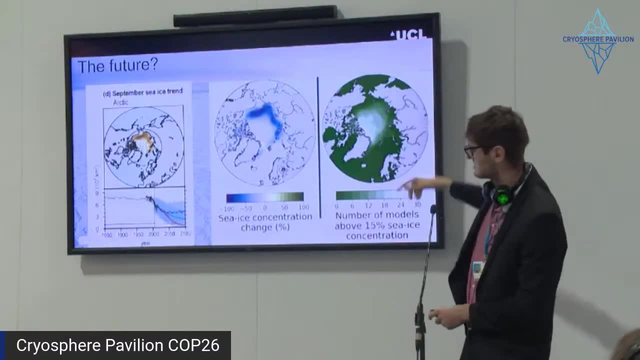 So that's a moderate emission scenario, And we're just going to see the same situation where the sea ice- over the next century to 2100, is going to retreat from the north coast of Alaska, the north coast of Siberia. 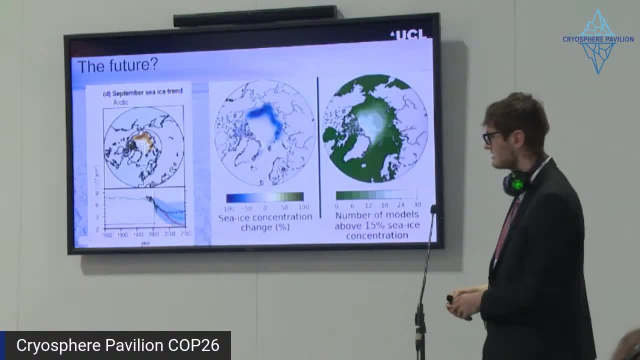 back towards what we call the last ice zone, which is north of Greenland and Canada, And on the left you can see the sea ice trend And in the bottom panel of the left hand figure you can see that the total area is again just very sensitive to the emission scenario. 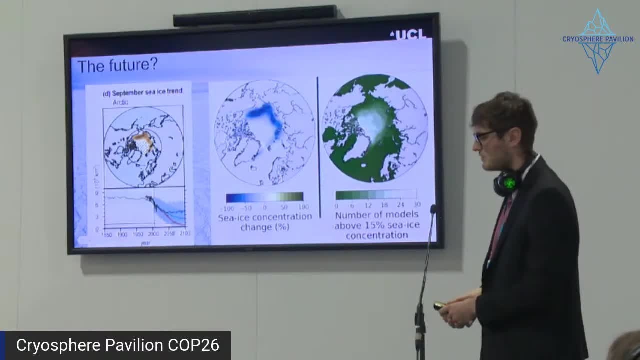 So the red line is a high emission scenario, the light blue a medium and the dark blue is the low emission scenario that would take us below two degrees of warming. So our emissions pathway really does dictate how much sea ice we'll see over the next century. 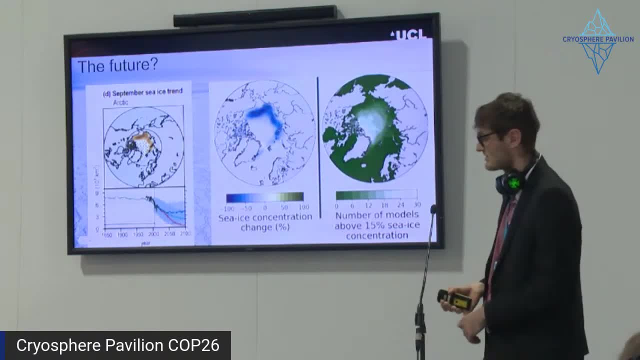 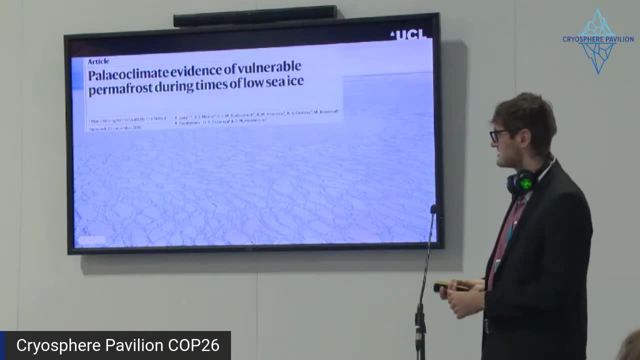 and therefore how much permafrost is exposed to the action of the atmosphere essentially. Finally, I just wanted to highlight some other studies that are very relevant to this. So last year there was a- it says received 2018, but it was only published in 2020.. 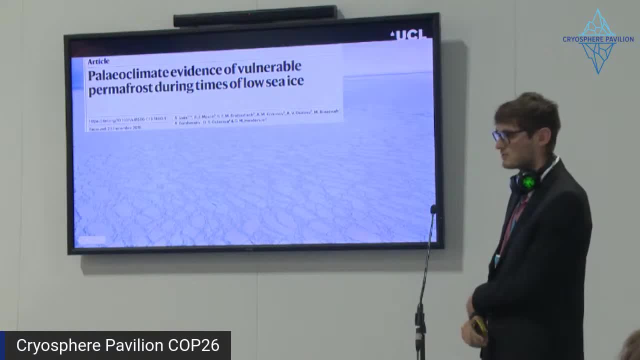 We had a paper that showed that as you look back in time at the permafrost in north Siberia, we really see that atmospheric temperature is not so much the dominant control but rather it's the sea ice extent, and Gustav's going to talk a bit more about that. 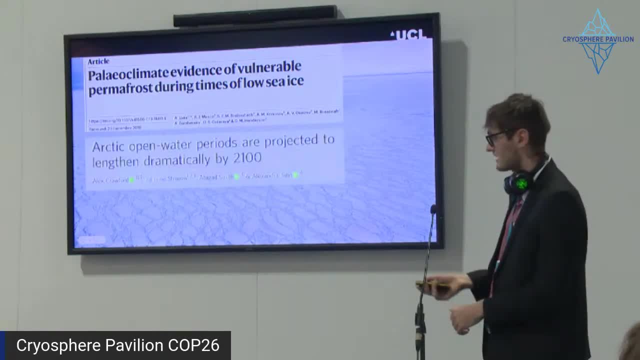 We also had this work that one of my collaborators and also my boss, Alex Crawford and Julian Struver worked on recently, looking at how the open water is going to increase, leading to increased permafrost exposure And finally, oh, and here is- the emission scenarios that actually lead to that increased open water. 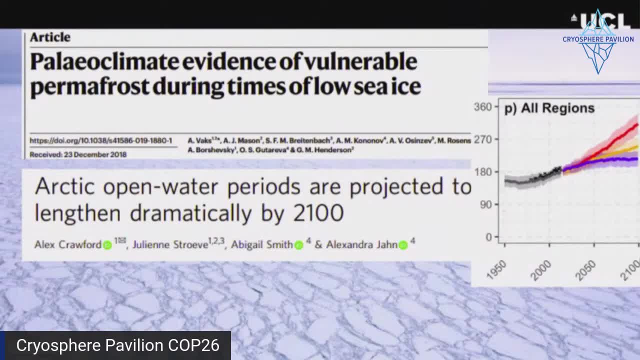 So, just like in the previous slide, I showed that our emissions really dictate how the total area of the sea ice is going to evolve. We also get to decide with our emissions pathway how long the open water is going to exist at the end of the century. 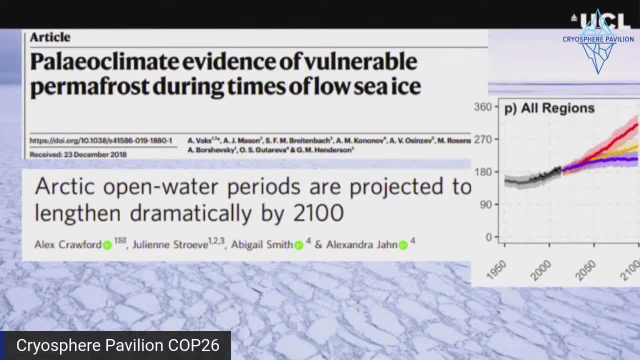 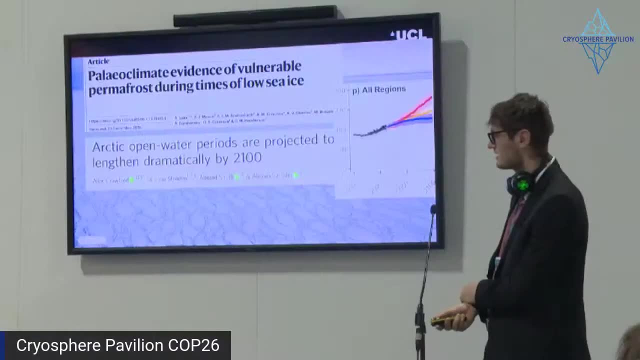 And again you can see, it's very sensitive to emission scenario, The high emissions scenario. we see over 270, more than 300 in fact, days of open water in the Arctic Ocean. So the duration per year of permafrost exposure is sensitive to our emissions pathway. 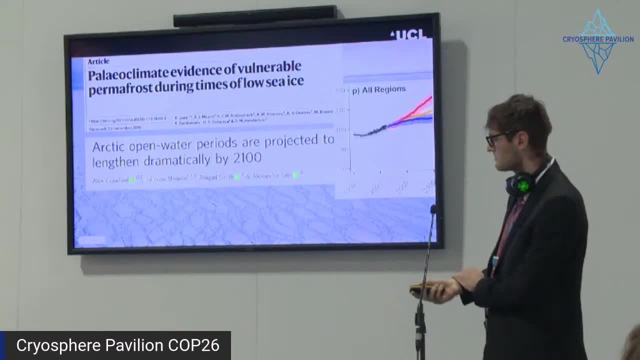 And finally, some work that's in review. It's not showing up on my slide clicker. Well, this is my last slide. It's not appeared, but we've got some work in review that, well, not we. there is some work that the community is currently reviewing. 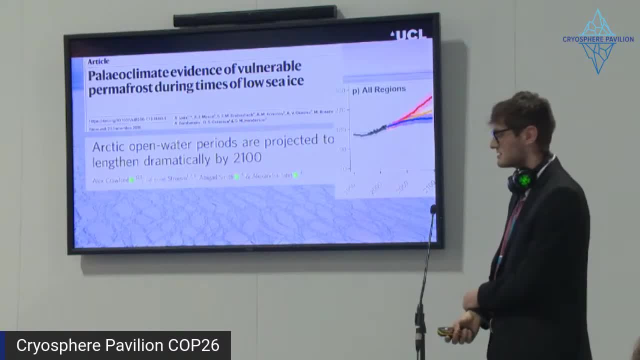 that shows that beyond 2100, into the 22nd century, the sea ice behavior still dictates the rates of permafrost thaw mostly through oceanographic changes. So I'm going to transfer now to Gustav Hegelius, who's going to talk about the more permafrost 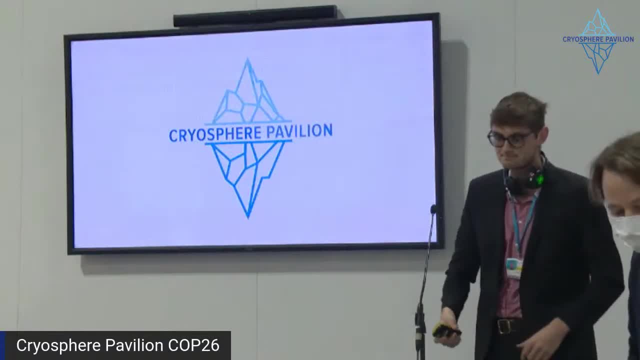 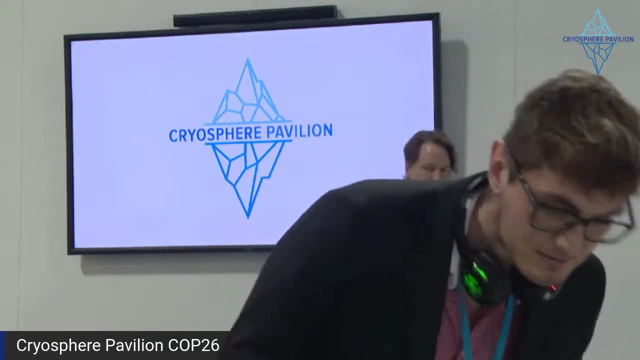 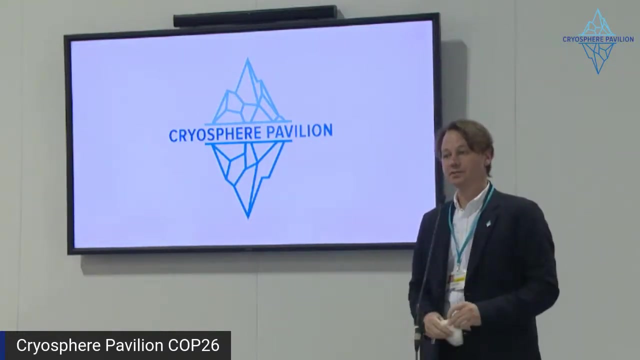 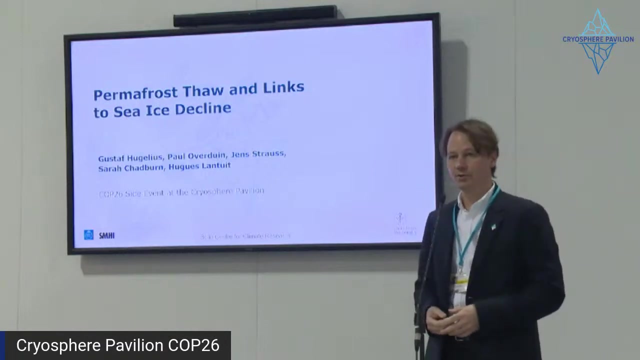 relevant aspects of sea ice decline Thanks. Thank you very much, Robby, for that talk. Also, that shows the sea ice trends and the drivers of this processes very clearly. So we're going to take questions at the very end of the session. 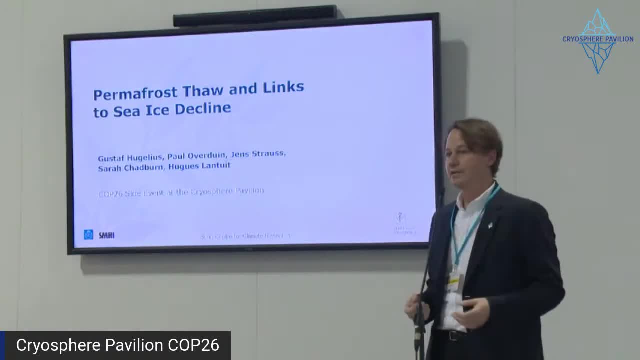 And then you can ask questions both to me and to Robby if you like. So this talk is then sort of following on the trends that we just saw. I'm going to talk about permafrost thaw and links potentially to sea ice decline. 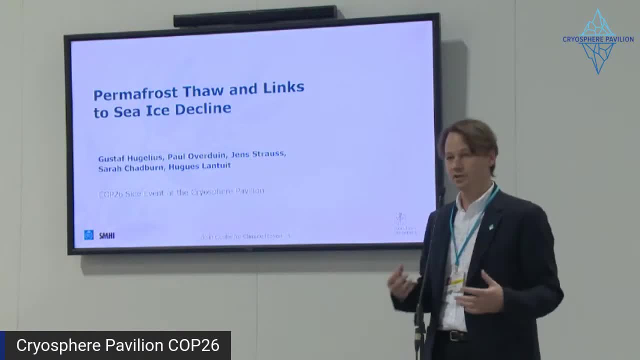 So I'm going to start with an introduction of permafrost thaw and the permafrost carbon feedback- for those of you that may not be so familiar with permafrost- And then I'm going to talk more tentatively about the different links that are observed in this topic. 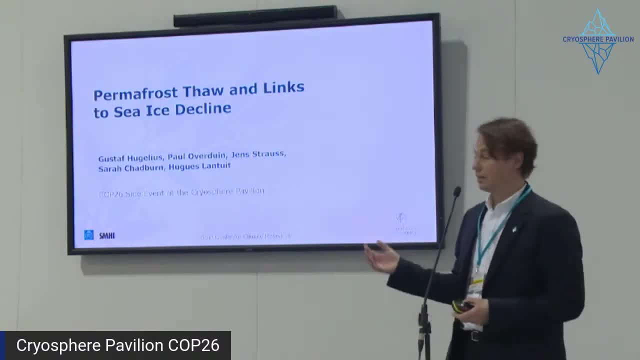 And I'm presenting on behalf of a lot of colleagues. You see my name: Paul Overdyn, Jens Strauss, Sarah Chadburn and Hyggeland Vy are all colleagues that helped us present on permafrost yesterday And I've taken material from different colleagues to put together for this talk. 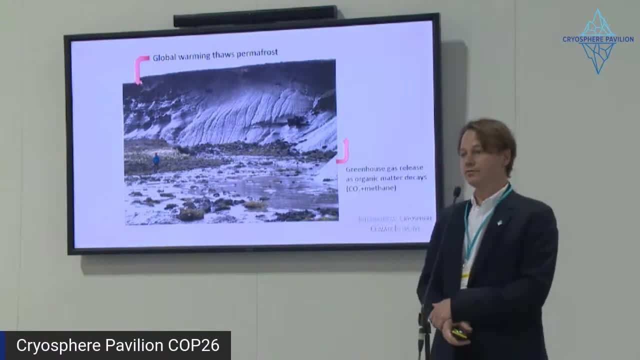 OK, but starting with really an overview of what is permafrost, Why should we be concerned with global warming affecting permafrost? Well, permafrost is ground that's frozen all year round. It's a very vast phenomenon: covers more than 20% of the land mass in the Northern Hemisphere. 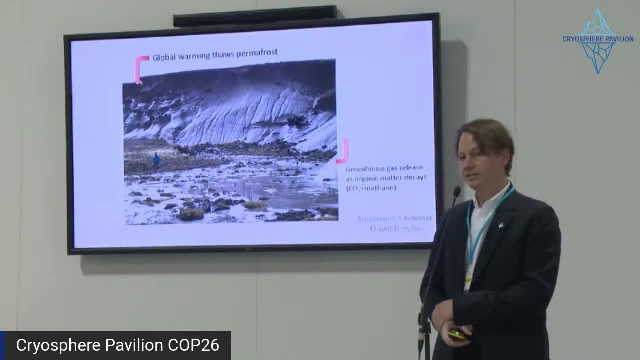 Permafrost is usually many, many millennia old and it has accumulated organic carbon remains, plant remains, for thousands of years, leading to a buildup of enormous stock of organic carbon. There's more carbon in permafrost than in the whole Earth's atmosphere and all living plants together. 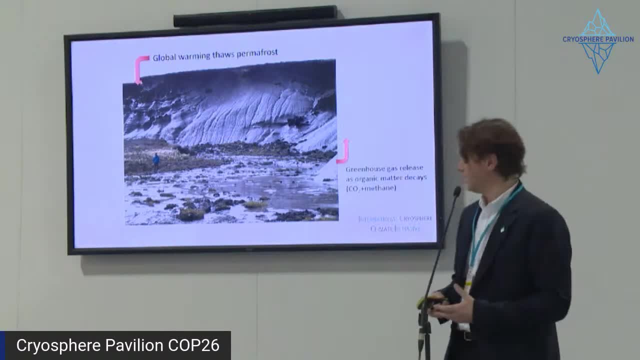 So it's about 1,500 gigatons of carbon locked in the permafrost region And when this thaws due to global warming, you can get very catastrophic sort of localized thaw events like the one you're seeing here. You see Professor Lantuy at the bottom left. 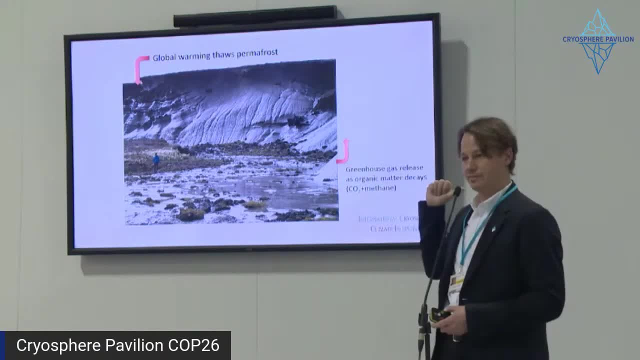 He's actually looking out over the ocean. So when I'm taking this picture, I have the ocean right at my back, on the Canadian Beaufort Sea, And you see a coastal cliff that's eroding in a thaw slump, exposing a lot of ice in the ground, a lot of organic material. 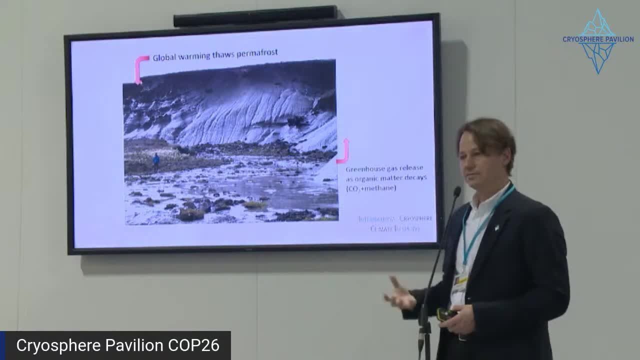 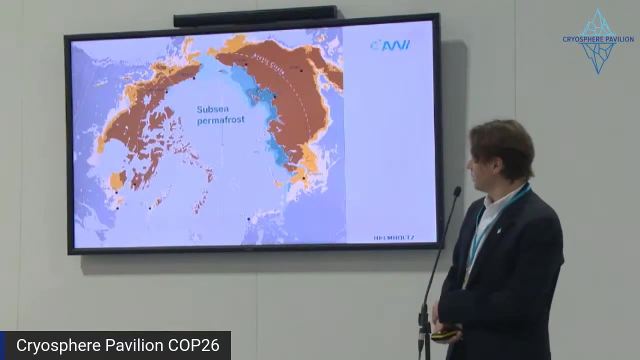 And when the organic material is remobilized, microbes can start to decompose. They basically eat up the old plant remains and they release methane or CO2 as a byproduct of their respiration. As I mentioned, permafrost is a vast phenomenon spread across the Northern Hemisphere. 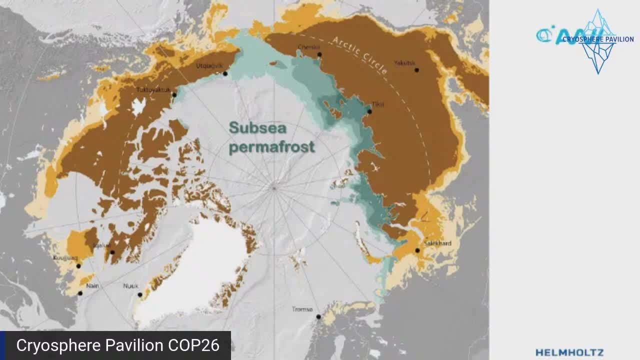 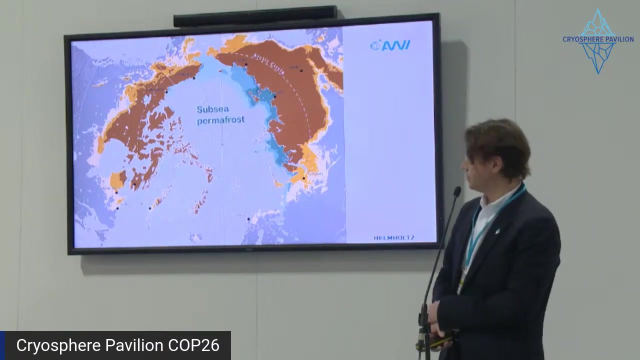 The orange part of it, the left of this map shows you terrestrial permafrost, And then the sort of green-blue colors show you the subsea permafrost that you already saw, what we showed you in the last slide. So this map is courtesy of Paul Overdue, Sebastian Westermann and Jaroslav Åbo and others. 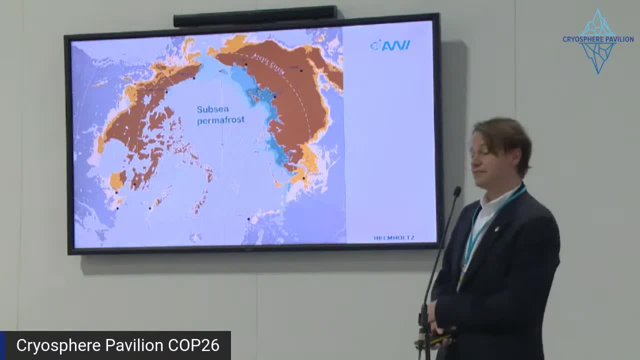 that have recently put this together, And it is, as Roby already pointed. it's a striking similarity between where the sea ice is declining most rapidly and where we have the subsea permafrost, but also where we have large extents of vulnerable permafrost on the terrestrial side. 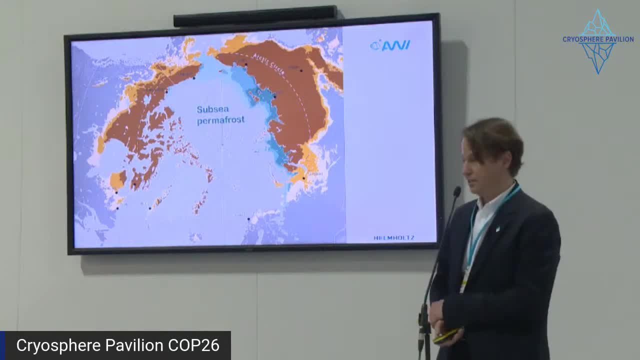 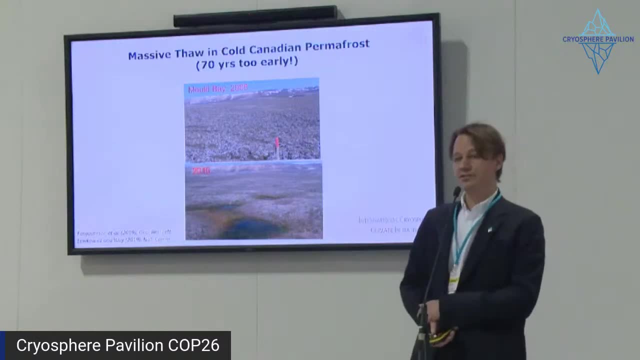 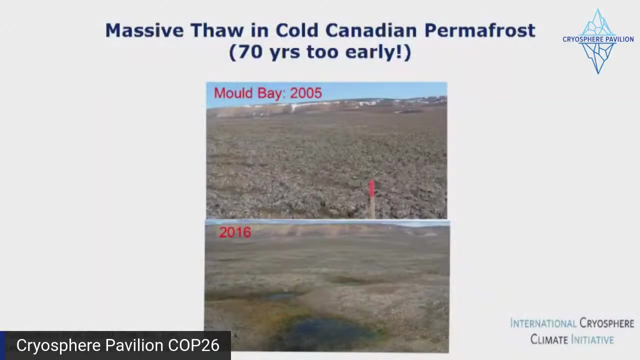 adjacent to the loss of permafrost area. I'm going to get back to this a bit more later. Unfortunately, we're seeing rapid and massive thaw of permafrost. This is an example from the cold Canadian Arctic, where a couple of summer heat waves 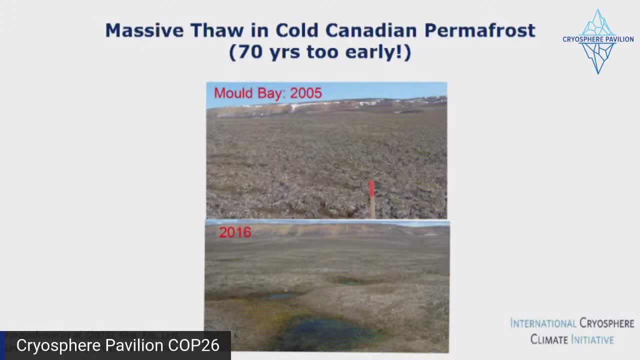 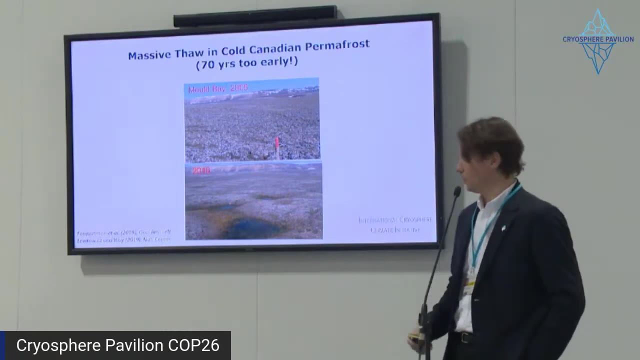 not the recent ones, but actually earlier, triggered abrupt thaw events where we actually see really fundamental landscape changes and abrupt thaw occurring 70 years earlier than it's supposed to occur according to our system models And if we look at extent of permafrost. 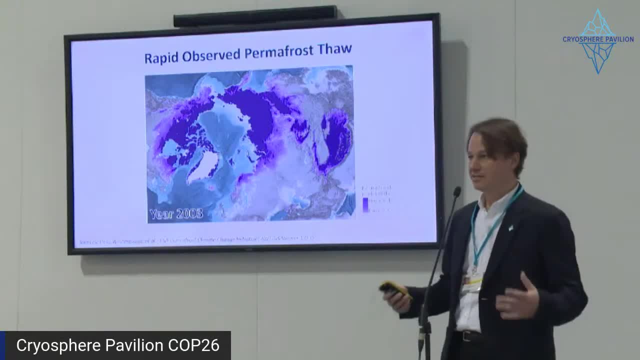 here you see, observed. it's a model driven by observation, So it's modeled. observed permafrost thaw. We're starting at the year 2003,. going to 2010, to 2017.. If I go back and forth a little bit, 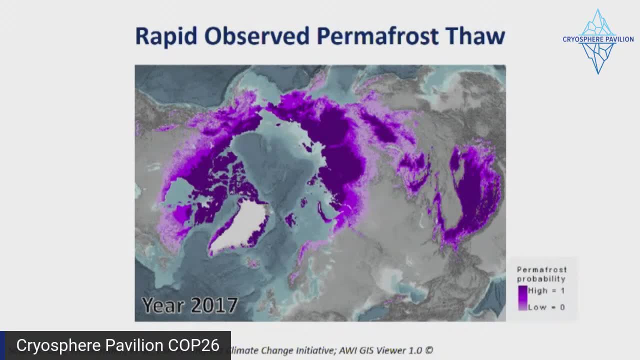 you see this very rapid decline in- and this is the very near surface permafrost. There will still be deeper permafrost in a lot of these areas. that is not lost at this rate, but this gives you an idea of the rapidness of the trends that permafrost is starting to thaw. 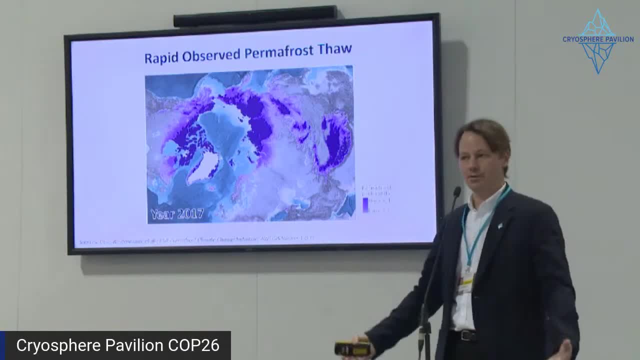 Overall, permafrost reacts very slowly. so the deeper permafrost permafrost can be up to a kilometer thick or even more. that will take a very long time to thaw. so these are the near surface changes that we're concerned with here. 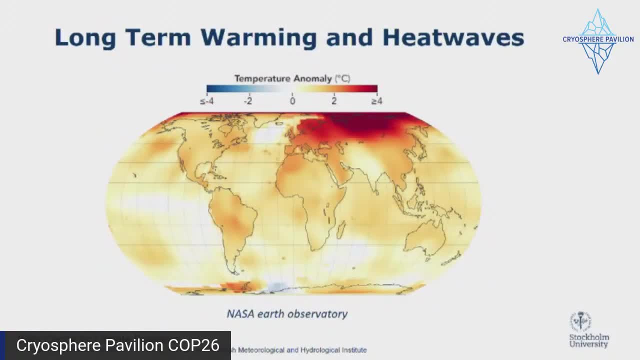 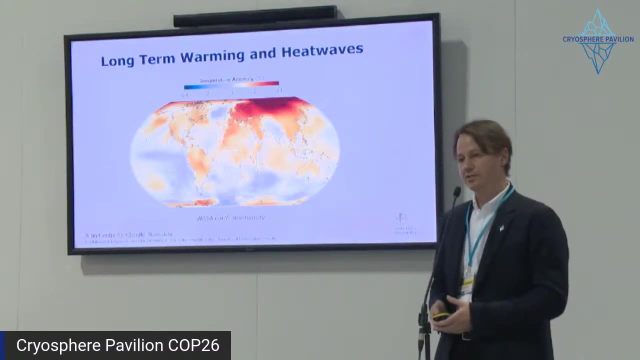 This is the temperature anomaly for the year 2020, and you see this massive heat wave that struck the Arctic And I note that it coincides really well with sea ice minimum in 2020 over the East Siberian shelf region. Of course, this points to regional linkages in the climate system. 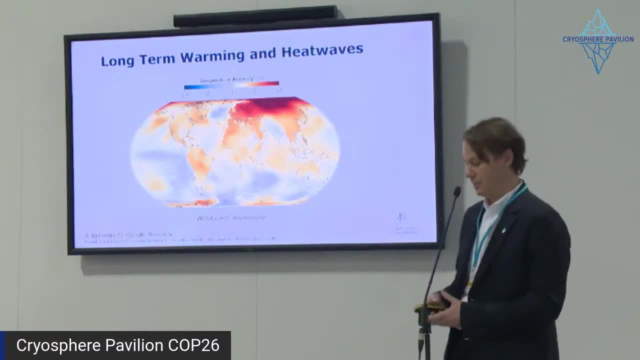 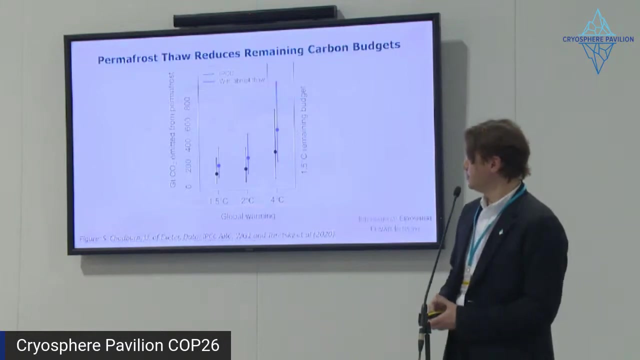 as well as, of course, as global changes to climate. But these heat waves are really striking at the heart of the permafrost region, where we have also the most carbon dense ecosystems within the permafrost region And permafrost thaw. 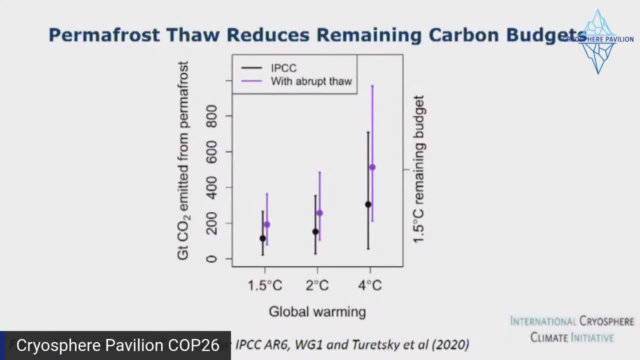 we're seeing a lot of permafrost thaw. We still haven't seen permafrost thaw accelerate to the point where the whole Arctic is shifting from a sink to a sink, from a sink to a source. It's right at the stage of the tundra is probably already a source. 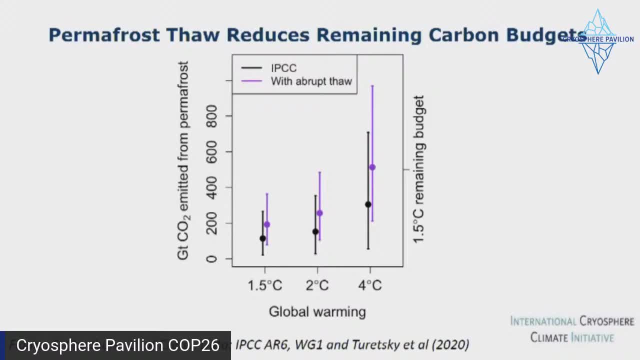 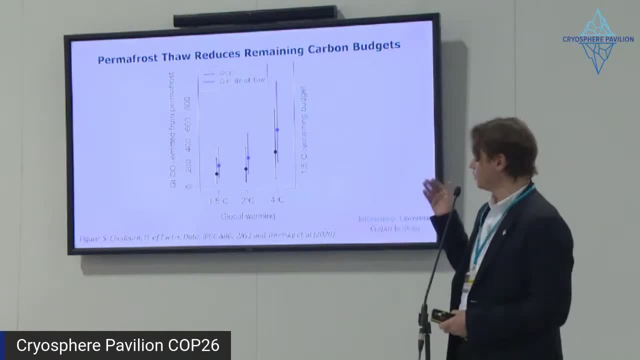 while the boreal forest permafrost is still a sink. But we're right at that transition zone And if we look at projections into the future, we're expecting this to really accelerate soon. So rapid permafrost thaw or permafrost thaw. 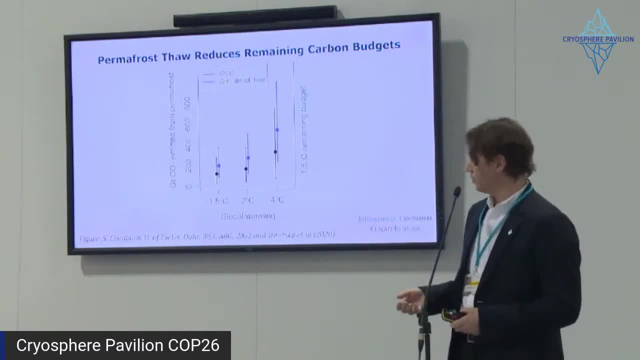 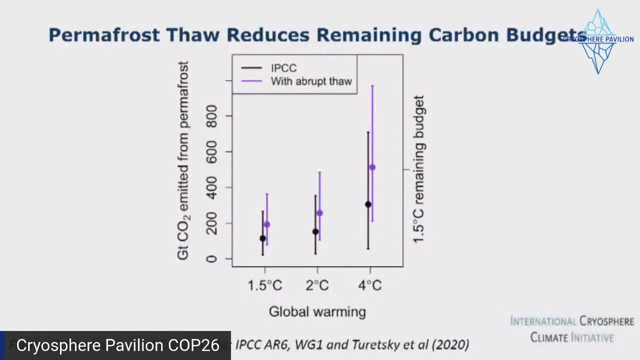 really reduces our remaining carbon budgets. This graph shows you gigatons of CO2 emitted from permafrost on the y-axis at different scenarios of global warming. You see what the IPCC included in the last assessment report and you see if we add processes of abrupt thaw from recent papers. 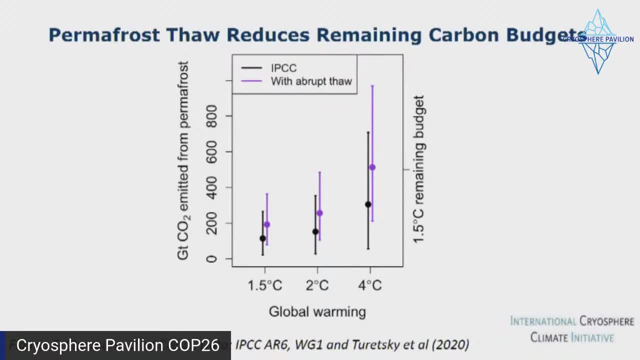 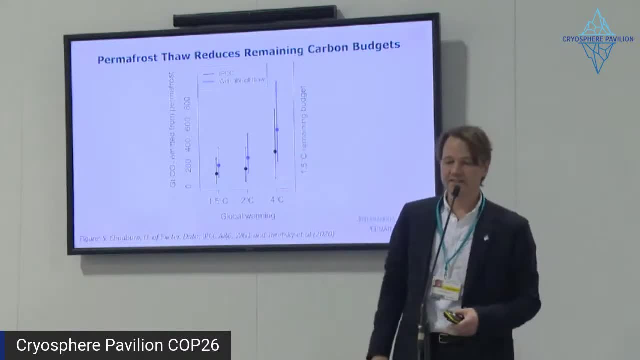 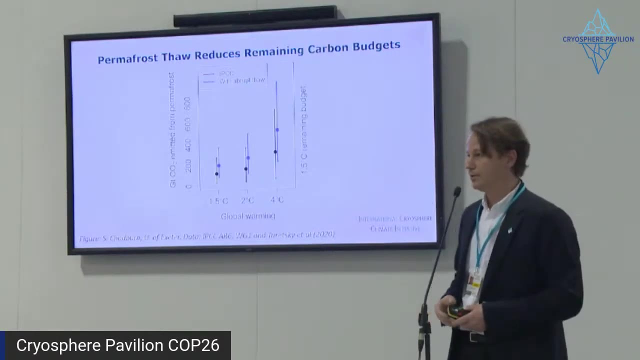 that weren't fully included to the IPCC report. These are very substantial emissions. You see, on the right hand side there you see the total cumulative remaining carbon budget to reach the 1.5 degree Paris goal. So the permafrost is eating up a very substantial part of that carbon budget. 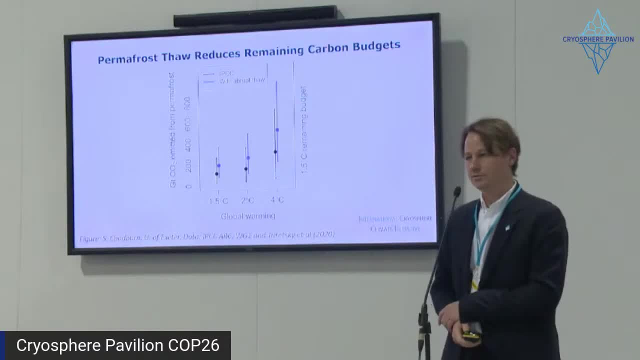 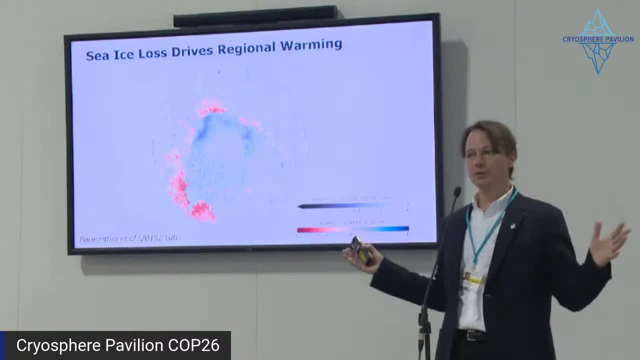 So these feedbacks also have to be accounted for when we're looking at our future emissions budgets. Okay, so that was the overall permafrost carbon feedback, And now I'm trying to zoom back to the linkages to sea ice. This is a graph from a paper produced by Frantz-Jan Parmetier. 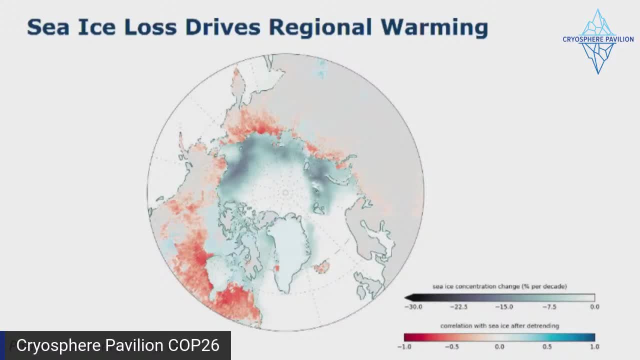 at Lund University in Sweden. He's done a lot of very relevant work on the linkages between different crises, different atmosphere components and especially looking at how sea ice affects the terrestrial ecosystems in the Arctic. So you see, this graph has two elements. 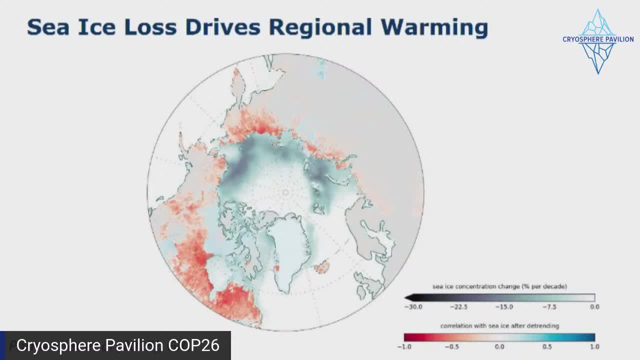 You see sea ice concentration change with the bluer colors showing areas where sea ice has declined, And you see in red correlations to increases, regional increases in surface temperature after deep trending. So this is having statistically tried to remove the general warming. how much of the warming can be attributed? 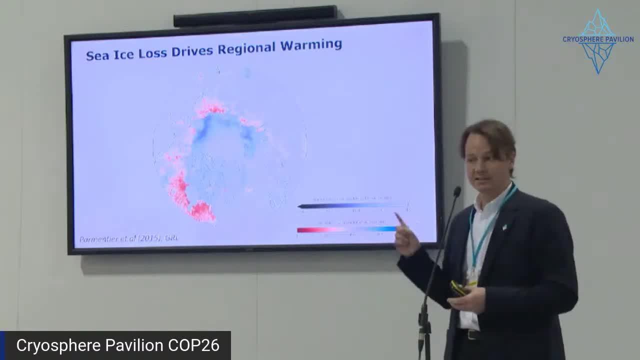 or is correlated with sea ice decline. A correlation does not always imply a one-way causality, So this doesn't mean that all of this correlation is actually driven by the sea ice, but it means that they are strongly connected. And yeah, so you see that there are actually 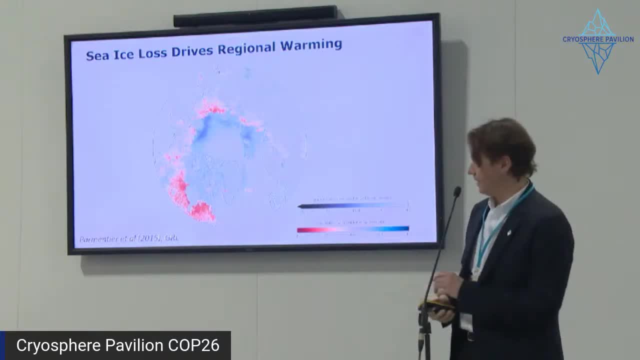 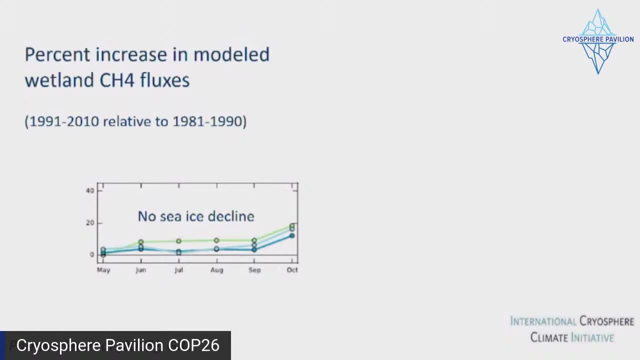 really strong effects in Siberia, really strong effects in Canada, And in this paper Franz Jan and colleagues actually showed, using models, how permafrost, or how sea ice decline, is linked to increase in methane release from Arctic wetlands. So one of the processes that is also tied to permafrost thaw. 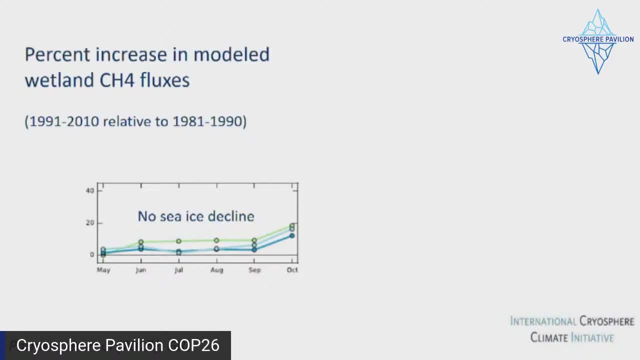 Here you see the relative increase in methane production in percent over the time period. in the areas where there was no strong correlation to sea ice decline. So basically, business as usual. well, global warming, as usual, I should say. you still see an increase, right. 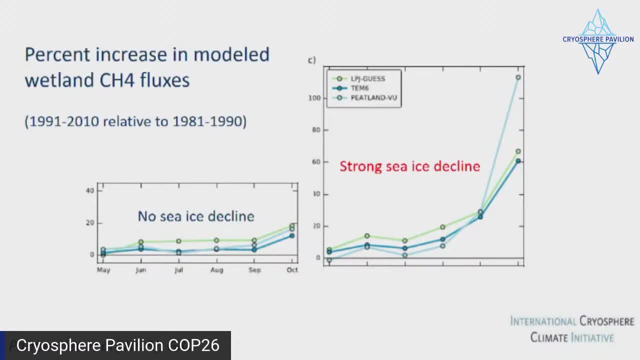 But then if you look at areas where there was a strong correlation to sea ice decline, the increase in methane production, especially in the late season when the sea ice is at its minimum, is enormous. So there is a really strong empirical trend here supporting basically direct linkage. 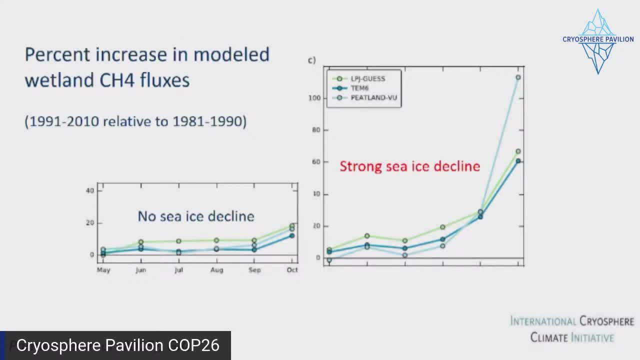 within the sea ice minimum and the increase of methane production. Methane production in general is you know it's very tightly coupled to the temperature of the environment where it occurs. The microbes are partially temperature limited, So this connection is quite easy to also link. 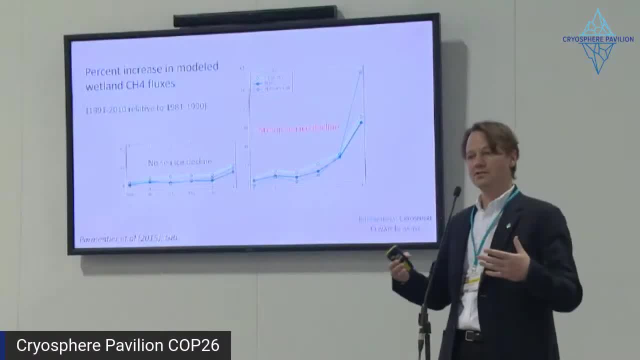 to our understanding of methane production. But of course temperature increase doesn't only increase methane flux, it also increases permafrost thaw. Those changes haven't really been fully triggered yet And they are explored in the literature, but I don't have a similar graph to show you. 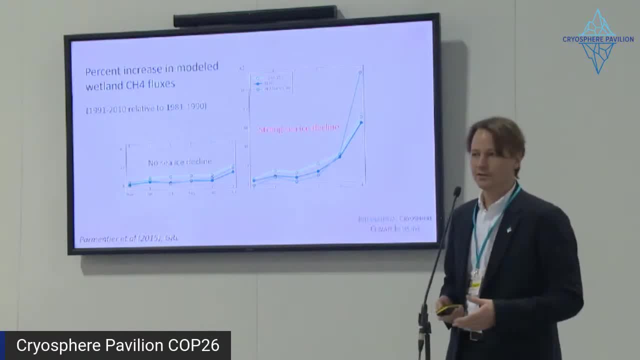 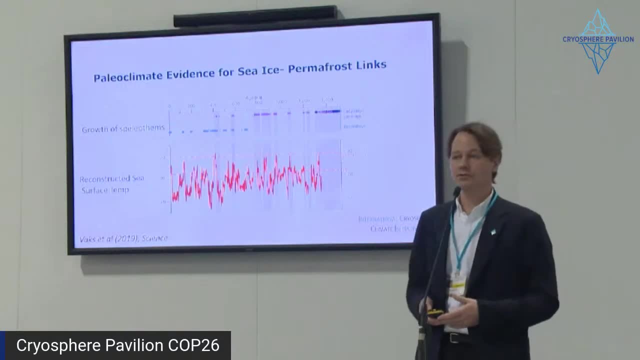 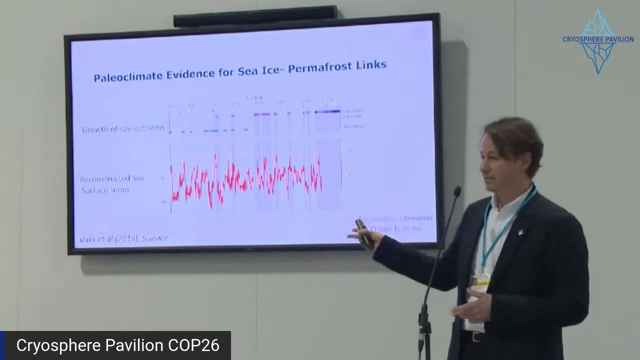 for direct correlation to increase permafrost thaw. Those processes are, in most likelihood, already occurring. I want to also show some evidence from another paper that we already Robbe already introduced us to this. It's from Vax et al, published in Science. 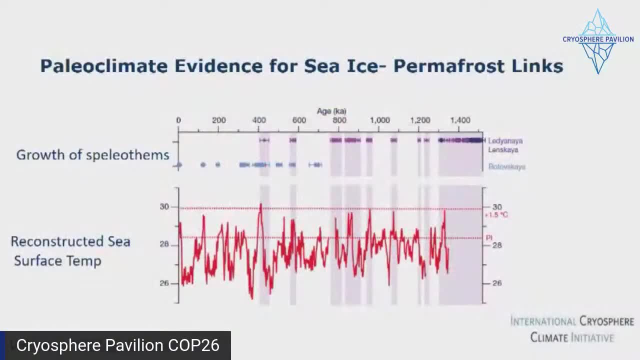 I actually have the wrong year. It should be 2020.. Sorry about that, But this is a really started taking a very, very long time approach. You see the time scale: it's thousands of years, So it's 1.4 million years. 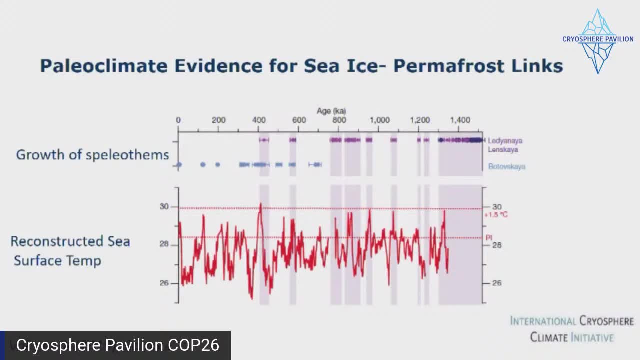 And they looked at the caves, at cave speleothemes, and they can actually recreate. so there's dripstones that occur in caves in different parts of Siberia And by analyzing the isotopes in those they can actually link the processes. 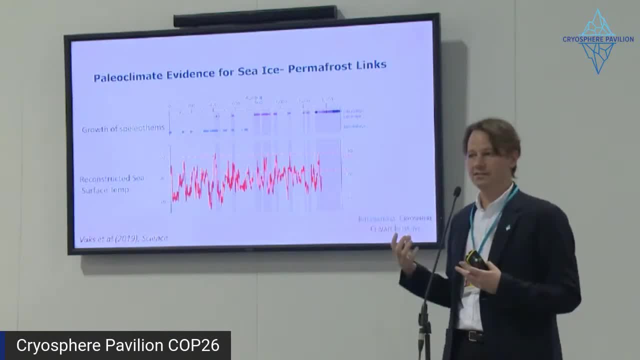 that happen on the surface with the formation and the growth rates of these speleothemes. So it's actually really cool You see the old, the really old permafrost being preserved or not preserved in these cave stones. So we actually 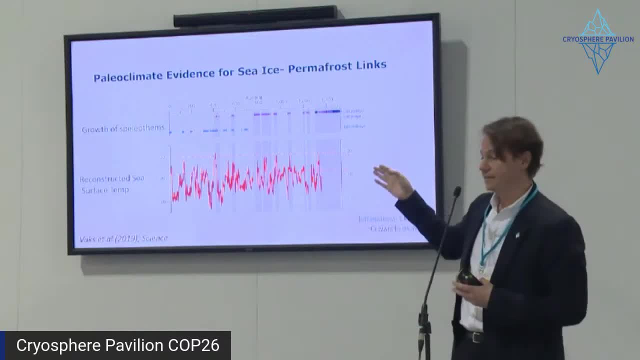 you have the growth of speleothemes on the top And basically, when the speleothemes are growing, there's no permafrost. When they are not growing, there's permafrost. So when the permafrost thaws, 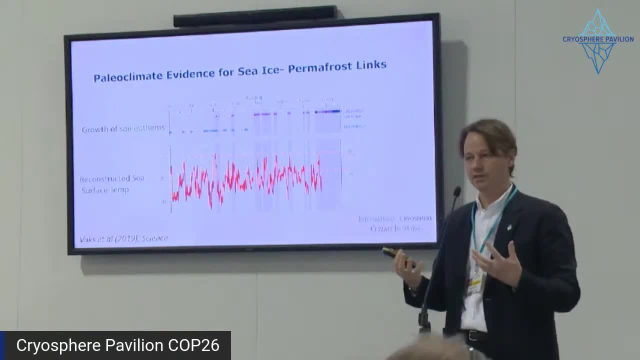 the water starts to come into the cave and the dripstones grow. When the permafrost is degrading again, when it gets colder, the growth of speleothemes stop. I think this is a. it's a really interesting paleo archive. 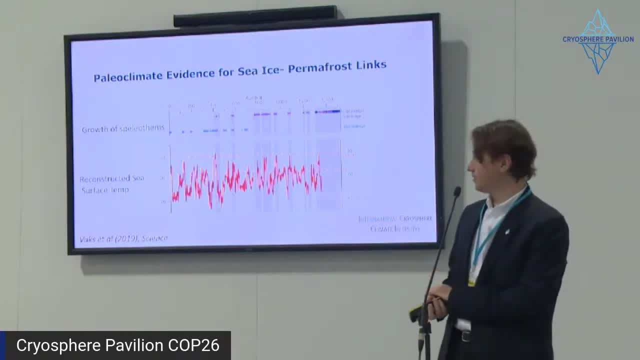 But here we just- they just show this in correlation to reconstructed sea surface temperatures And you can see quite a lot of agreement in this of sort of deep time speleotheme growth with reconstructed sea surface temperature And you also see a very clear connection. 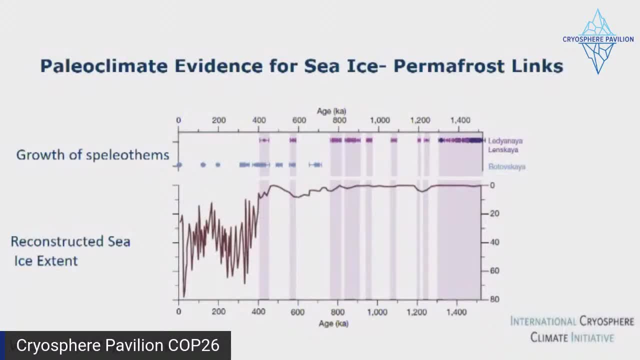 to reconstructed sea ice extent when we start to get into a colder climate after 400, after the 400,000 year mark, where you go from basically no sea ice to quite a lot of sea ice. So they're able to show these quite nice linkages between sea ice. 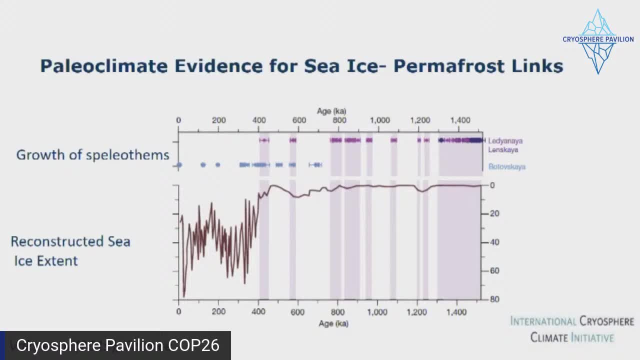 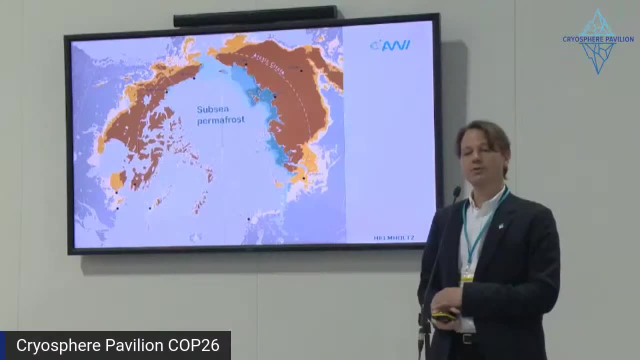 and permafrost stability at very long time scales as well. So this is something that has happened before, And I want to get back to two other processes that are also relevant. Now we're moving from land into the sea, So when we're crossing from land into the sea, 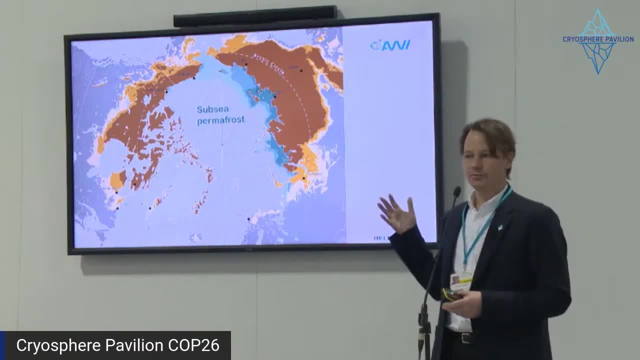 we're sort of passing the permafrost coasts. And permafrost coasts are also really vulnerable to erosion and to thaw, not just from climate, but also from the side, from sea action, from waves basically, And of course. 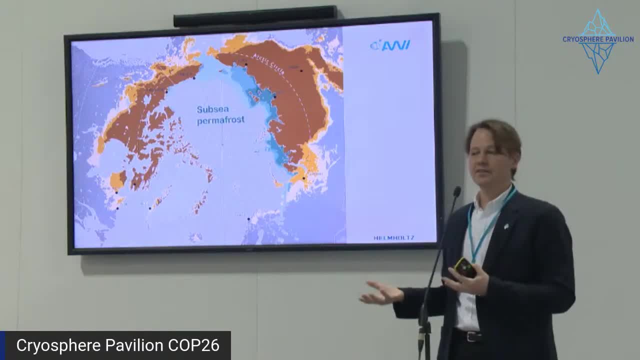 the wave action is very suppressed when you have a lot of sea ice And when the fetch, which is the distance the waves can build, increases as sea ice declines, you get a stronger coastal erosion And notably, if you look at this map, 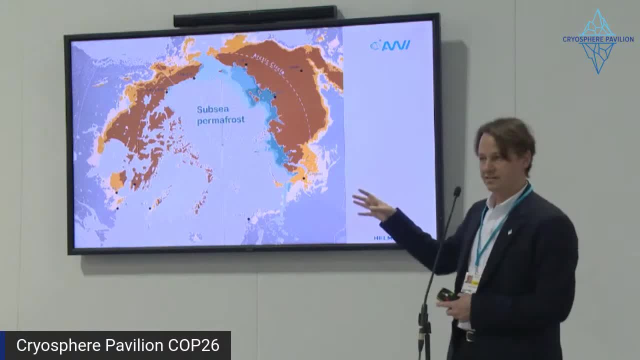 of the permafrost region. the areas where the sea ice is declining, also coincides with areas where the permafrost coasts are made out of sediment. They are not lithified, They are not bedrock. They are sediments that are just held together by permafrost. 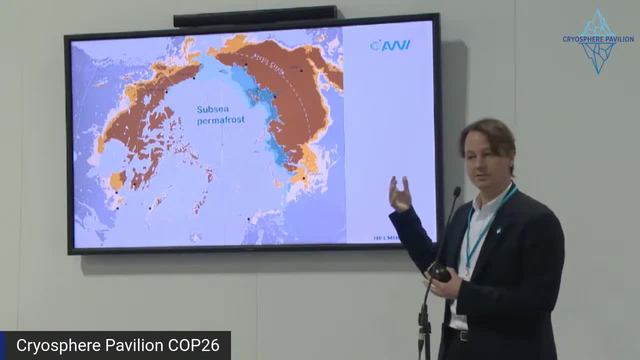 So in the areas around Greenland and northeastern Canada the coast is bedrock mainly. But if you go to Siberia and the Beaufort Sea area, the Beaufort Coast in Canada and Alaska, the Mackenzie Delta region, it's all sediment coasts. 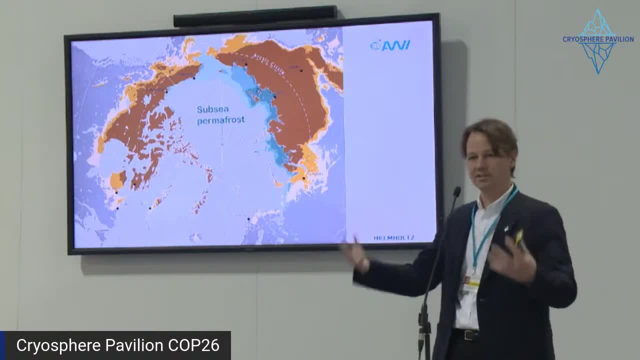 And that's also where the sea ice is declining and where the coastal erosion intensity is growing. So this is yet another feedback, And there was Professor Lantoui from the Alfred Wiggin Institute who had a presentation here yesterday where he just showed one example. 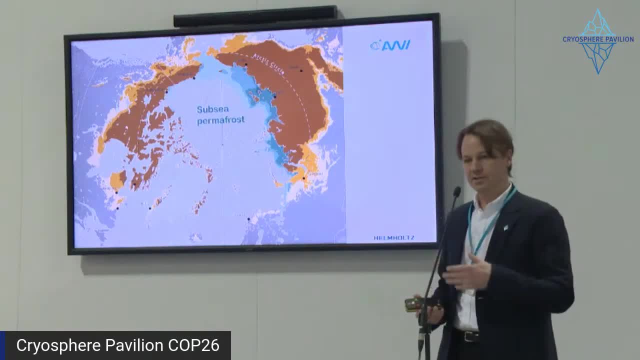 from the Beaufort Sea, where they've seen the coastal retreat increase from 0.4 meters per year to more than eight meters per year in just a few decades, And there's a really strong correlation to sea ice decline in this case as well. 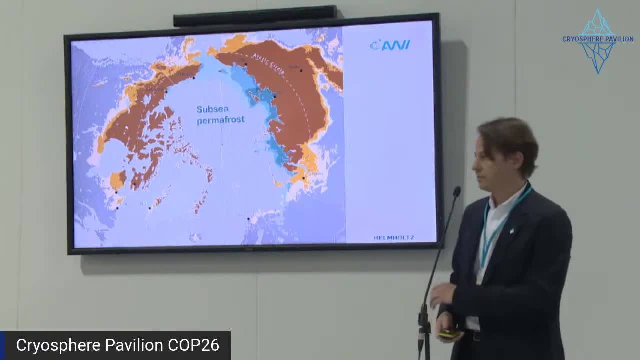 They see almost a direct correlation to the fetch in this increase. So that was the coast, And then we're moving out on the coastal shelves to the subsea permafrost Again. you see this in blue here Again, the areas where sea ice decline. 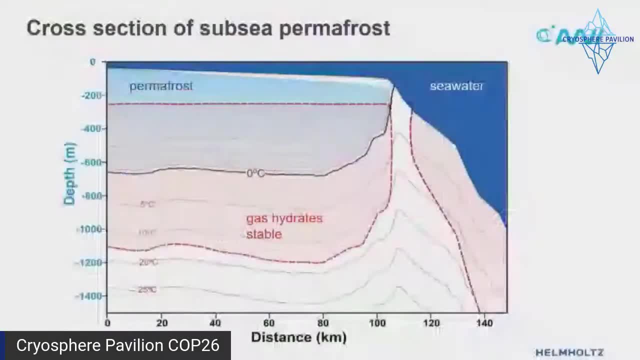 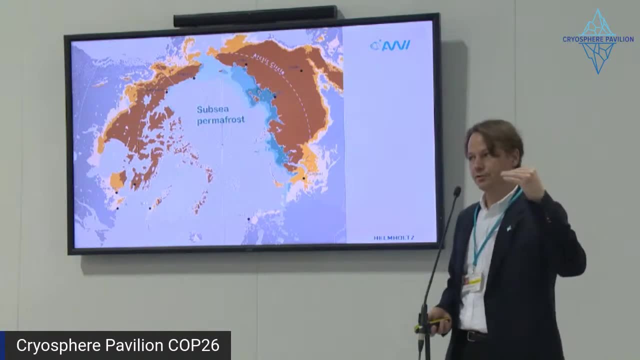 is the most rapid. Now, I'm Sorry I go back again. I'm going to go into sort of a transect looking at the permafrost system from the side. The transect is based on actual data from the Tuktoyaktuk. 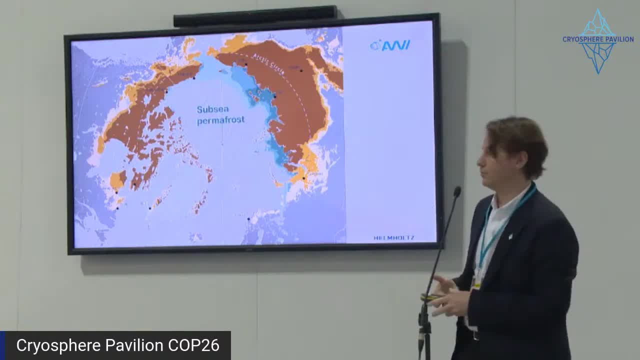 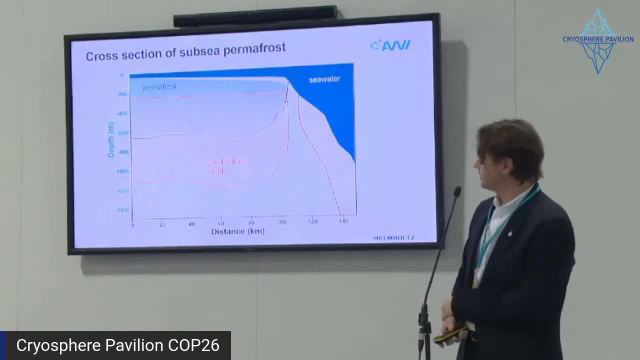 or outside of Tuktoyaktuk in the Canadian Beaufort Coast region Up there And now we're looking at a cross-section of subsea permafrost And there's a lot of elements to this. You see seawater in deep blue. 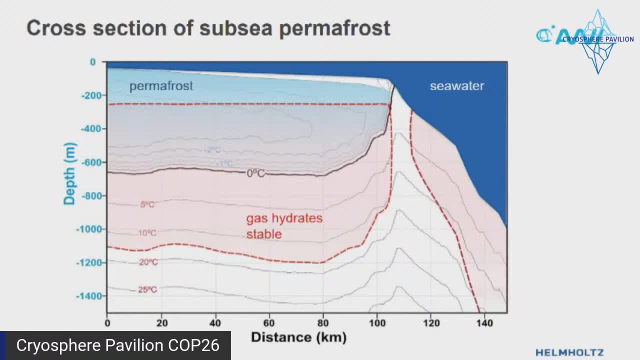 You note that the continental shelf is very shallow and then you have a steep decline to the deep ocean And you see in light blue, you see permafrost. Most of this permafrost actually formed when the continental shelf was not under the ocean. It was exposed to the atmosphere during the last glacial maximum Because when we had a lot of ice sheets on Earth, more water was tied up in ice, which meant that the global sea level was lower. So at the last glacial maximum, 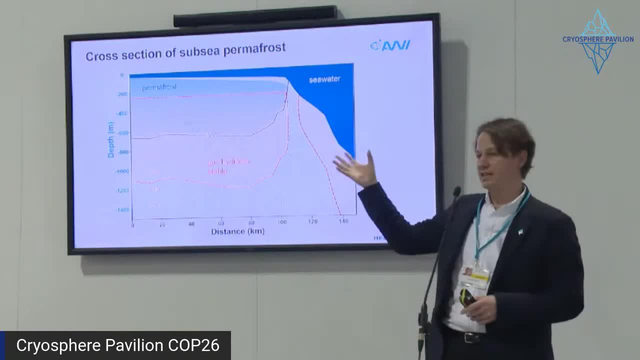 the sea level was there, Meaning that the whole shelf was exposed to the atmosphere and permafrost formed, actually in a terrestrial environment. And then we came out of the glacial cycle and it was submerged under water. And, as you can see, as soon as it starts to be submerged under water, it starts to thaw. Water is a very effective at sort of conducting heat, and also the salt in the water interacts with the permafrost etc. So the subsea permafrost would be thawing even without climate change, But it's going a lot faster. 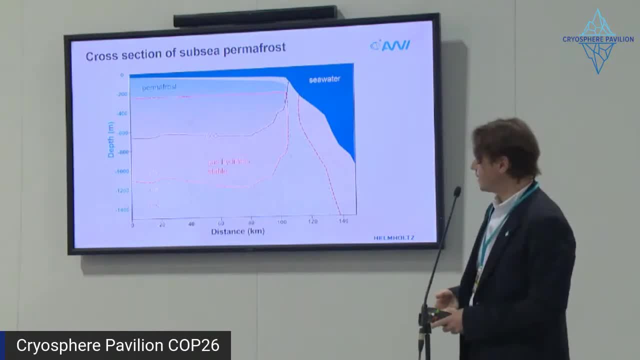 with climate change. obviously- And I want to talk about just mention the last component of this slide that's in the red- The gas hydrate zone. And gas hydrates are basically you can think of them as liquid gas that forms under very specific conditions. 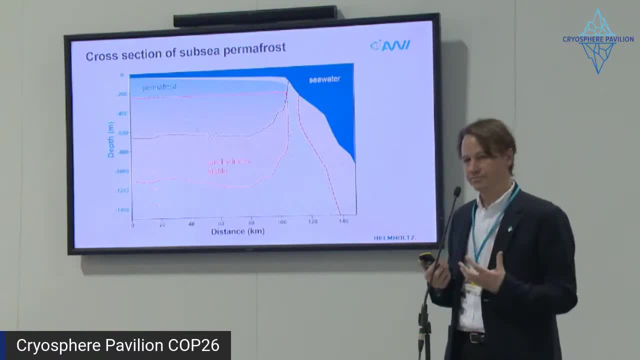 of high pressure and low temperatures, And these are often containing basically pure methane, And you have these zones where the gas hydrates are now stable but as permafrost thaws they would start to become instable and it can actually also be. 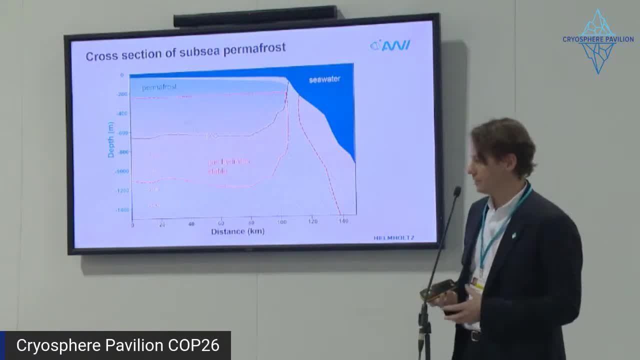 it can be released as bubbles or that reach the atmosphere directly or into the water column. But the interesting thing about the connection to sea ice here is that one you know the shelf seas used to be covered by sea ice and now they are to a large extent. 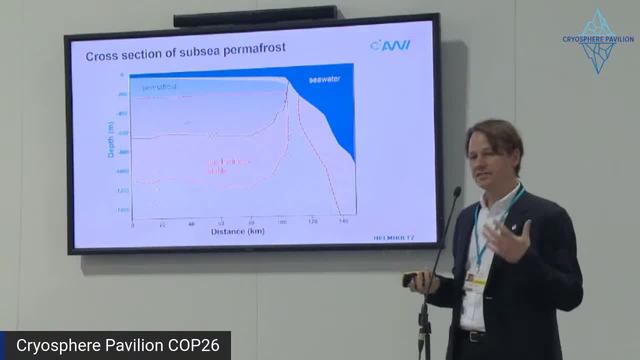 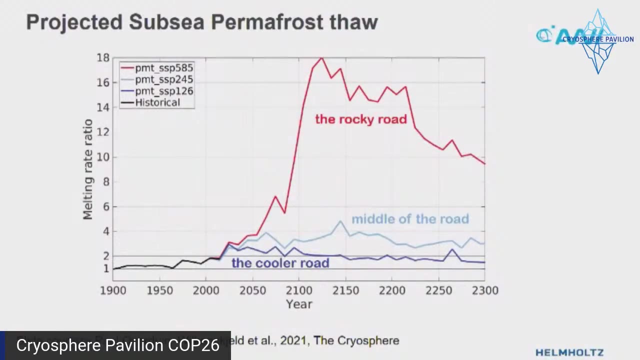 not covered by sea ice for a big part of the year And this has been shown to actually correlate quite well to the decline of the subsea permafrost. This is from a very recent paper that is really sort of novel work in being able to model subsea permafrost thaw. 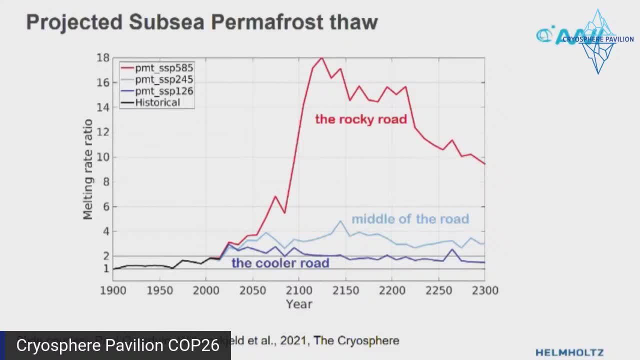 coupled in an earth system model. You see the reference at the bottom. Again, slides courtesy of Paul Overdune. This was the last ones before. It's from his talk that he gave yesterday And you see the different scenarios: the rocky road of high warming. 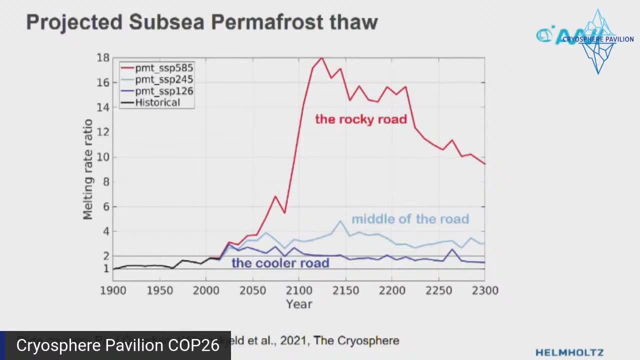 middle of the road and the 2.6 scenario, which is called the cooler road here, And you see this enormous runaway thaw of subsea permafrost happening in the rocky road scenario, And what this actually corresponds to very well is in this model. 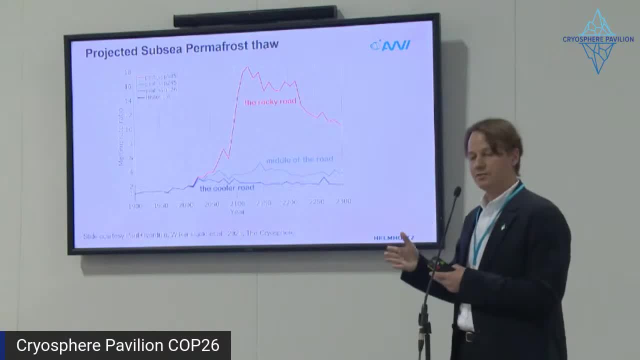 that is, when sea ice, when there's a threshold in the model, when sea ice basically disappears or it's almost completely gone, And then the model shows us very strong feedbacks between ice, freeze ocean and rapid thaw of the subsea permafrost. 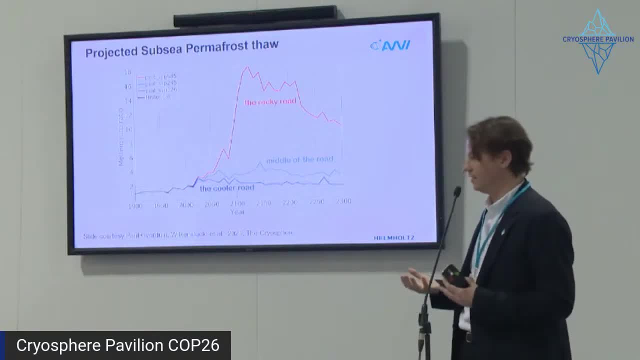 This is not at all fully explored yet. It's quite indicative. You know it's still early days And you know there's a lot going on, But the hypothesis that I talked to Paul about it yesterday and the hypothesis they have, is that once the sea ice is gone, you don't have any more formation of brine, which is this sort of very cold, salt-rich water which sinks and then actually keeps the brine formation from the sea ice, sinks and keeps the bottom water colder. 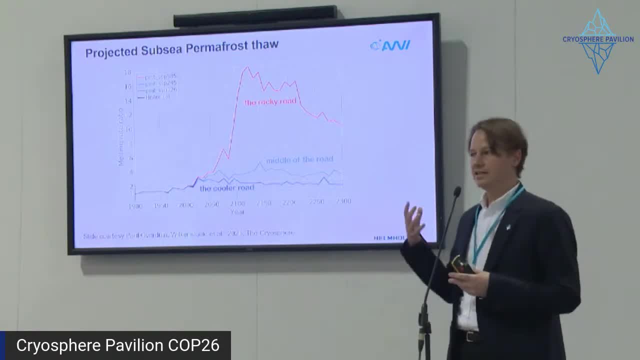 Once there's no sea ice, there's less brine formation. They think that this is what's driving the very rapid loss of the subsea permafrost. So there's this quite direct linkage between the sea ice, potentially, and the subsea system. 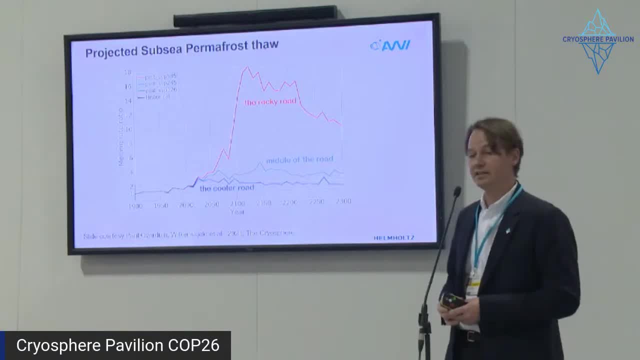 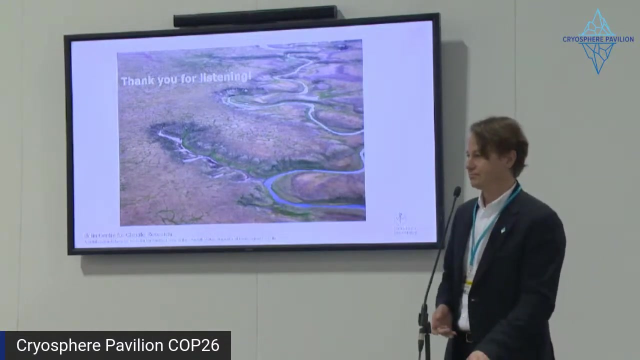 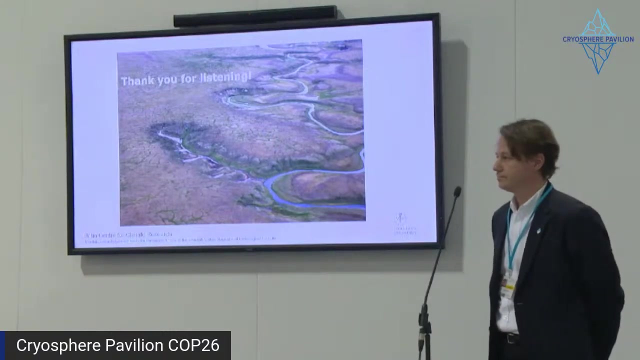 which is a very concerning, very interesting scientific finding, but extremely concerning when it comes to the potential climate response of the subsea system. Yes, thank you. That was my last slide, So thank you all for listening. If there are any questions, 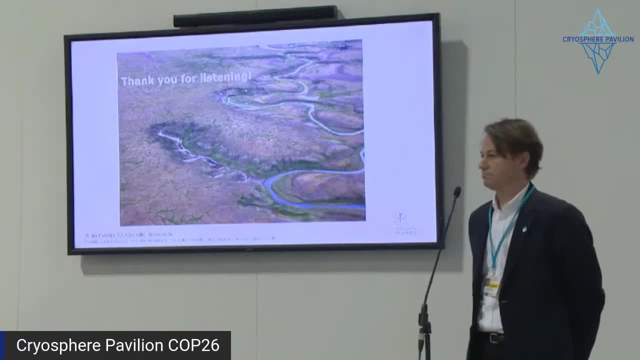 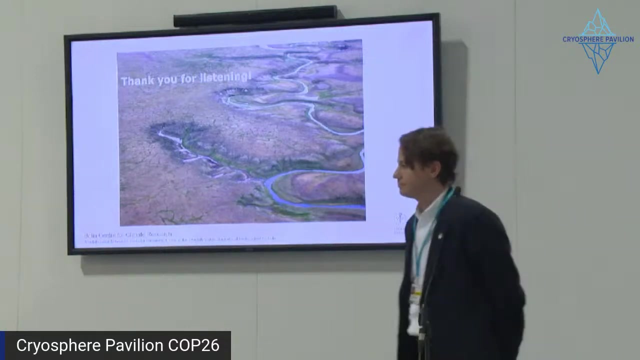 we can take them at this microphone. Are there any from online or from the Stockholm or the Geneva hubs? Okay, Robbie, do you have any commentary? Okay, One question from me, then. What do you see as the most important next research step to better understand these? 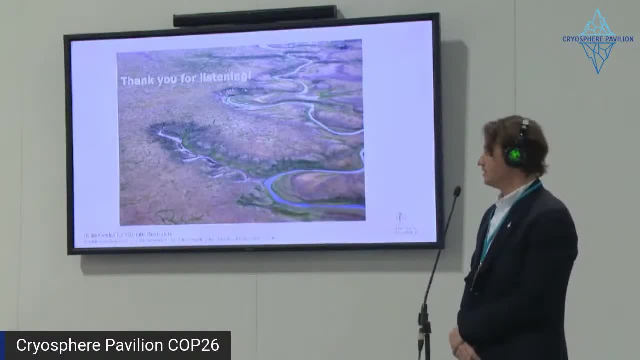 Thank you. So yeah, that's a good question. I think that the linkages to the terrestrial ecosystem have been shown for, for instance, when it comes to methane flux, But I think we really need to look at the sort of more long-term connections also. 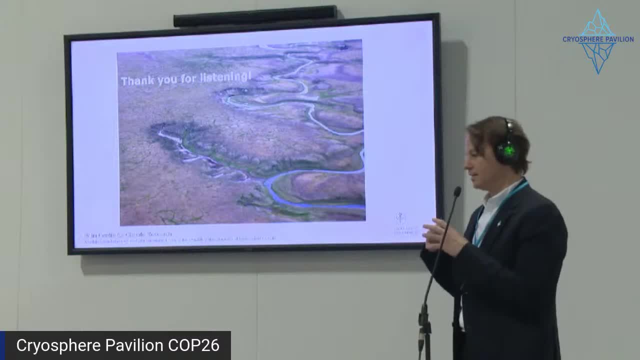 in having additional warming, additional regional warming driven by sea ice loss, actually incorporated into a coupled model that can really also quantify and isolate the feedback from the direct regional feedback from sea ice loss to the permafrost system. I mean it's implicitly already there. 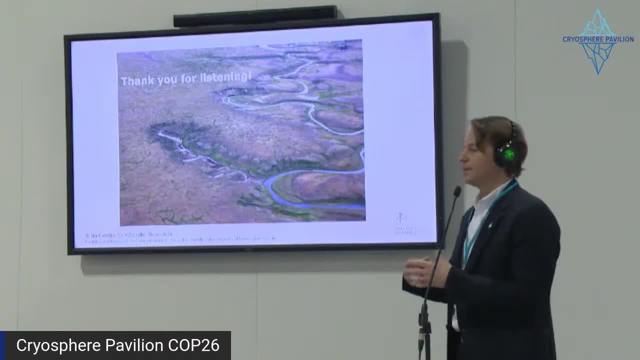 in the general amplification of warming in the high latitudes. But I think you know the evidence from Franciane's work suggests that there are more direct linkages as well, related to like precipitation feedbacks and other things as well. So I think we need to better. 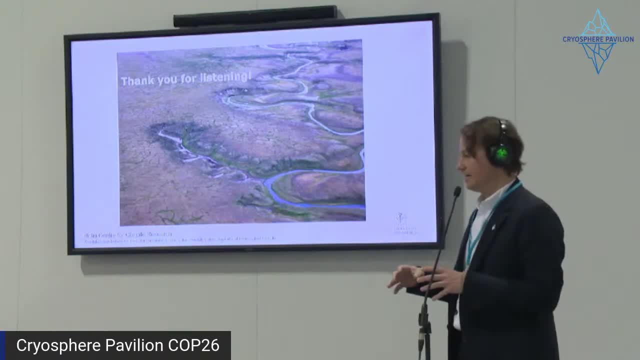 in coupled models, really understand the linkages. And then I think, when it comes to the, the work on subsea permafrost, which you know, I only learned of yesterday. this is extremely interesting And I hope that you know. 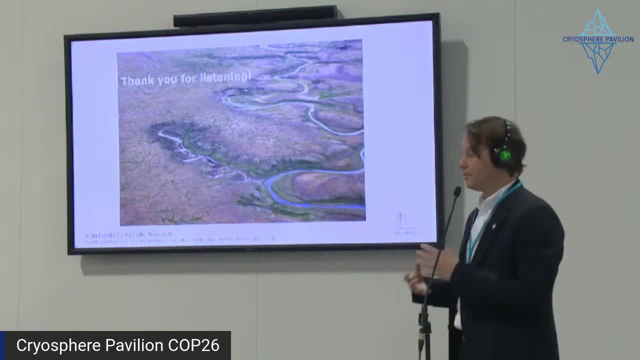 the groups working on this will really explore both the you know, really finding the mechanisms behind these, these feedbacks, and also be able to sort of better, better quantify the links between between the sea ice extent and the subsea permafrost. 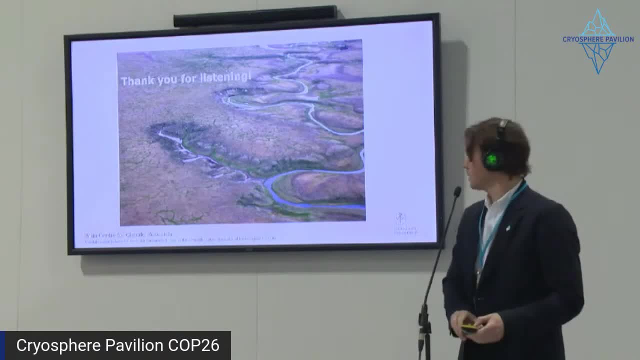 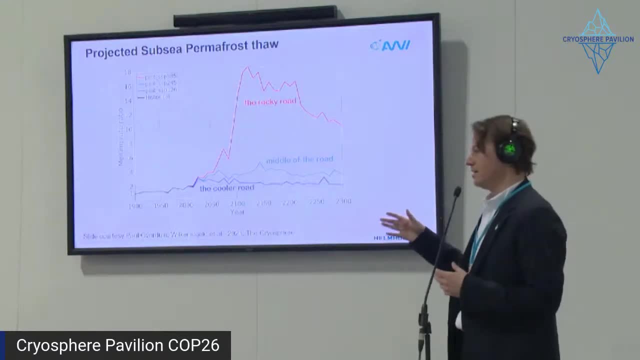 Because I also think that the Earth System model that they use- now I'm going to back up the Earth System model that produced this result- doesn't doesn't necessarily have the sea ice dynamics right. So I think the sea ice loss in this Earth System model. 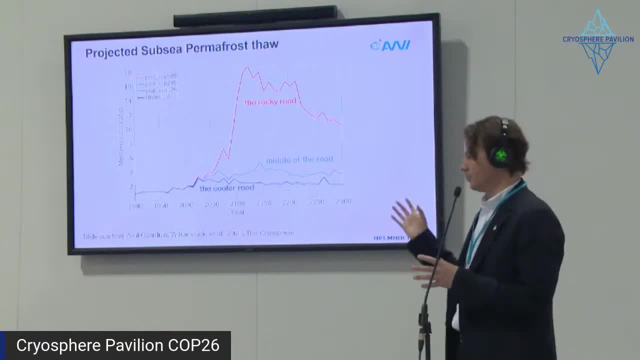 is actually happening a little bit later than what, more than what models that are better at sea ice modeling would would project. So it could be that, you know, perhaps sea ice loss is even more rapid than what this model suggests and that the timing will even be different. 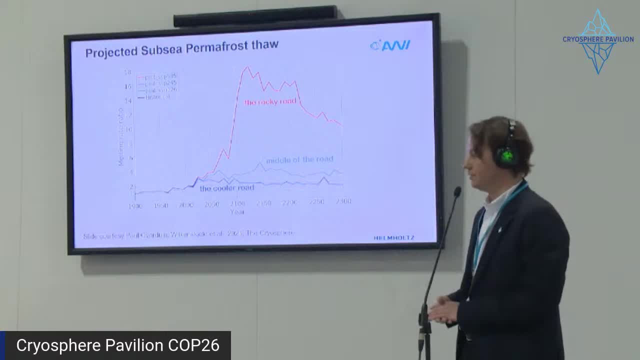 So I think there's pursuing this, this, this further is, you know, very interesting. I guess that's a a follow-up question then. Yeah, Cause I was noticing that the melt ratio but no temperature. So I know that scientists hate to speculate. 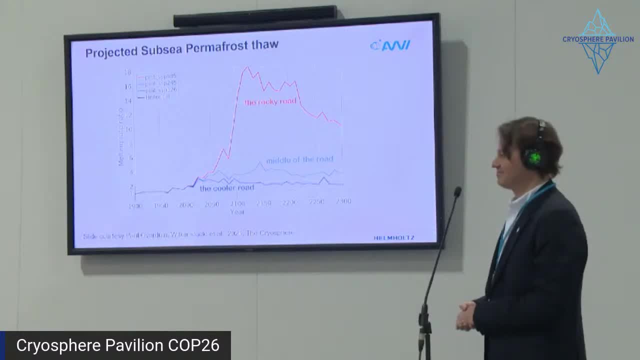 particularly for you, maybe subsea permafrost rather than land. but okay, let's say that we exceed this approximate 1.7 degree threshold for summer sea ice loss every year- That's going to be spoken about later on today- And then manage to take temperatures down below 1.5,. 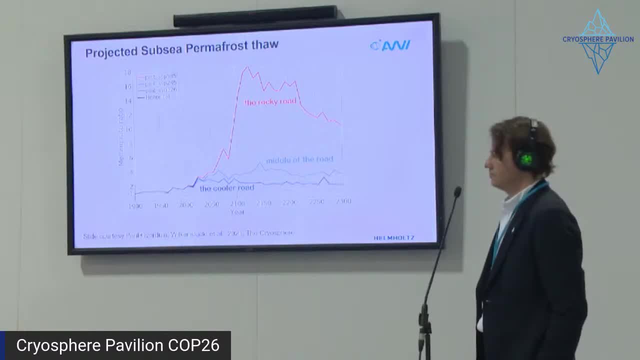 where there are occasional ice free summers, but not every summer. How fast do you think the system would respond to restoration of sea ice? Oh, that's, that's a good question. I to, and I have to be honest, I really don't know. 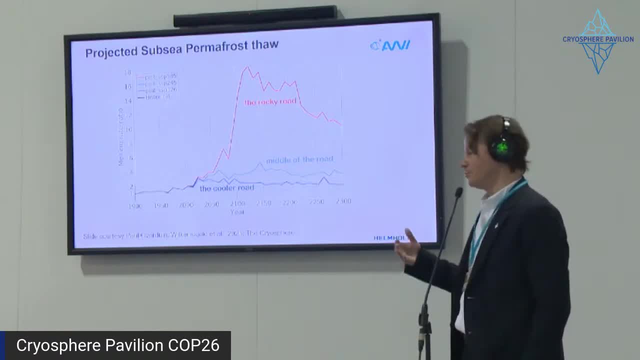 I really don't know the answer to that, but I mean, I think the the the sea ice system has the capacity to regrow faster than the permafrost system. Permafrost is extremely slow in responding to everything And I 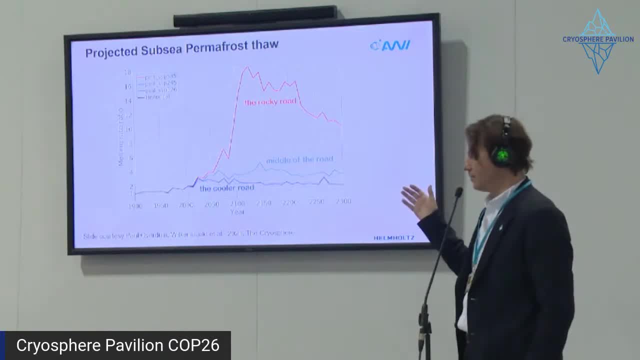 and I mean just looking at this, it it seems like there might be a threshold behavior in the subsea permafrost system in response to this. If it's really as fast as this indicates, that's, that's really, you know. 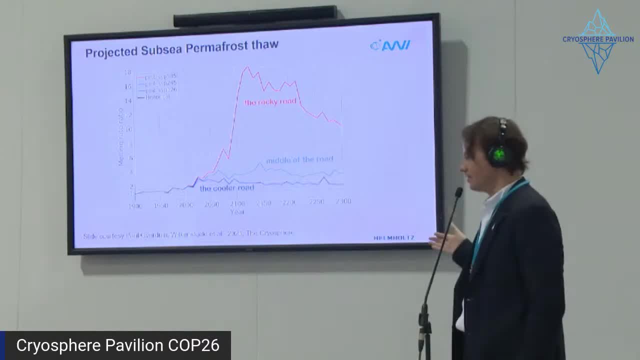 that's really concerning. But it might also be that you know, if the response is slightly slower, that you can avoid really triggering that that threshold by pulling, you know, by regrowing sub or sort of lengthening the, the 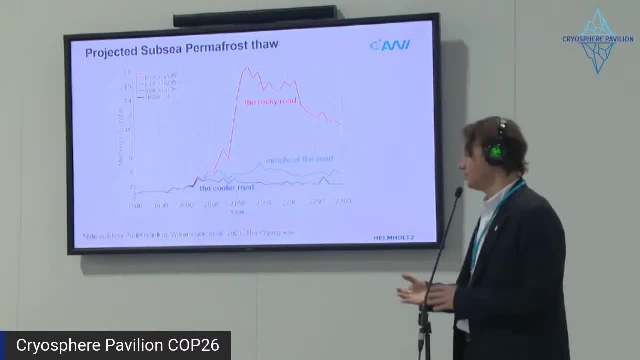 the sea ice season again. But it's it really. yeah, it's. I mean, it's a concern for completely that's unknown, to me at least, but very concerning. Thank you for being willing to speculate just a little bit. 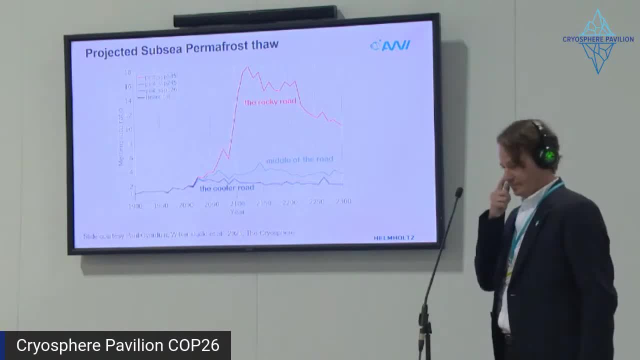 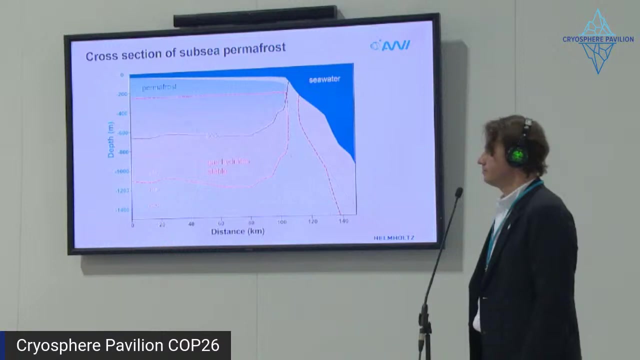 Any other questions here in the room? Yeah, please. Thank you, You mentioned there was a gas hydrate zone that has lots of methane locked into it. When do you anticipate that being uncovered and releasing that? What sort of time period are we talking about? 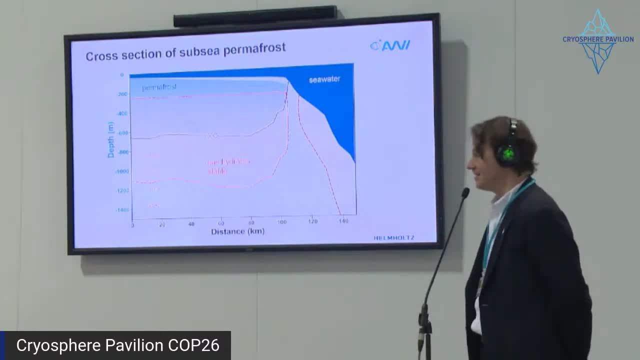 I? I'm really not qualified to answer that question. I think it's. it's something Paul Paul presented on this yesterday and it's it's extremely uncertain. I think there's some observational evidence suggesting that part of this zone is already. 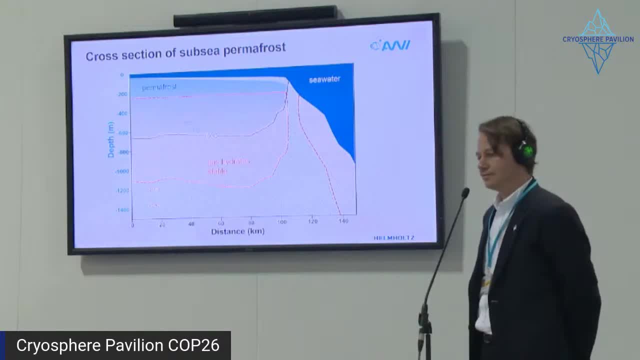 being active on the slope, But I think there's a lot of diverging scientific opinions on this And it's, it's, it's. I have to, you know, stress that I'm I'm an expert on terrestrial power plots. 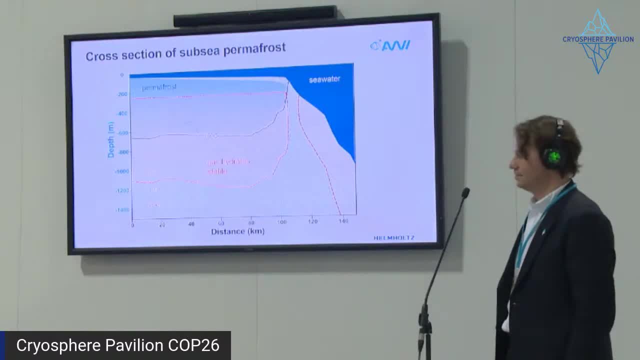 So this is really not not my, my, my kind of expertise. The paper that came out maybe six months ago that looks like it was gas hydrates on land in Siberia. This was from limestone caverns, I believe. I don't know if that's the same thing. 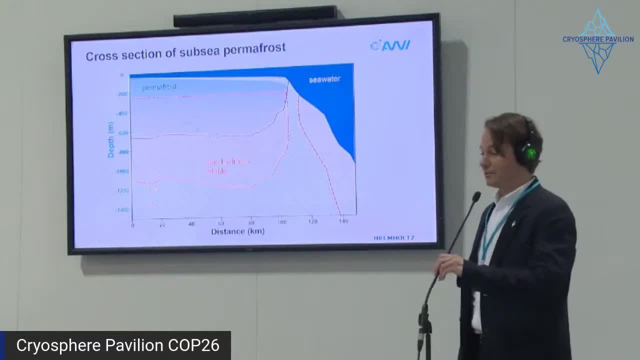 but can you speak a bit to that, maybe I? I'm not super familiar with that, but it's I, I'm yeah, I'm not really read up on that, I'm sorry, yeah, Yeah, Any other questions? 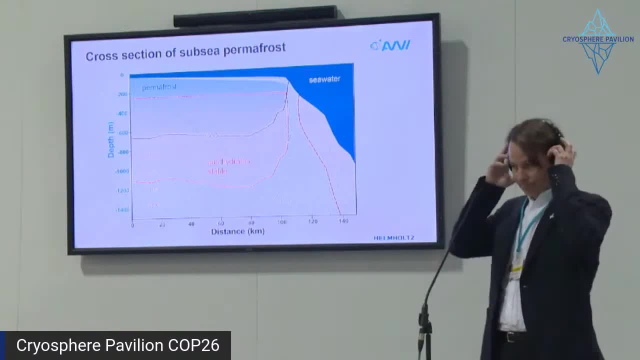 Okay, Thank you so much. Our next event will be be on the future of Arctic sea ice at 1 pm. thank you so much.